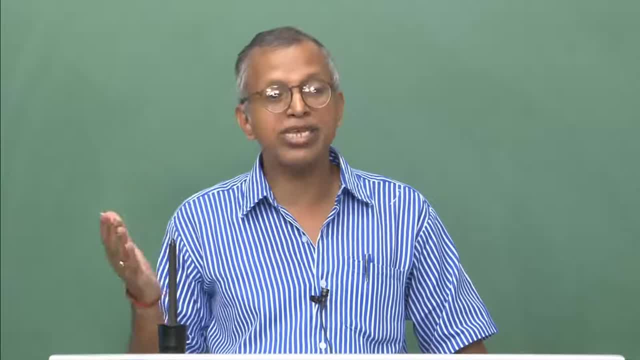 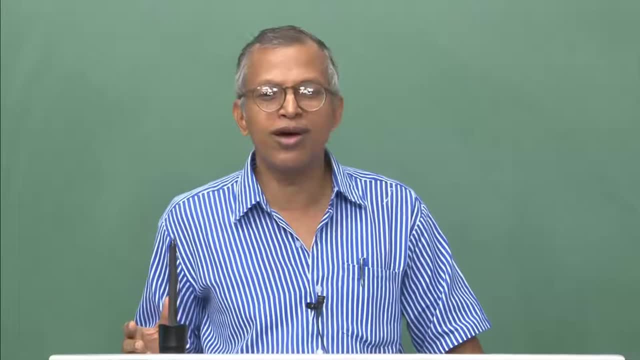 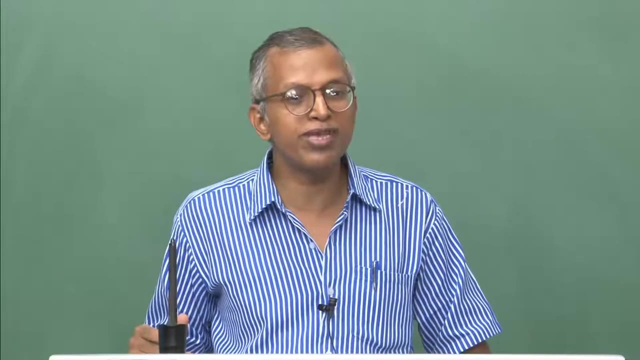 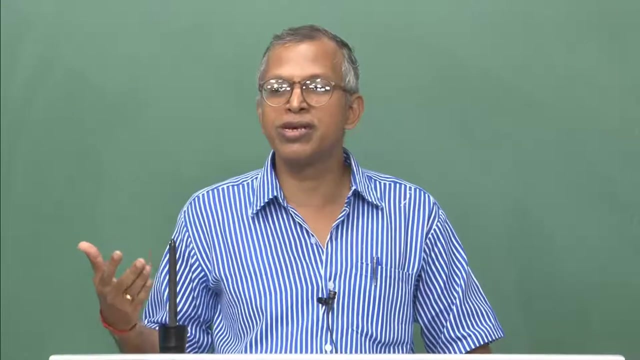 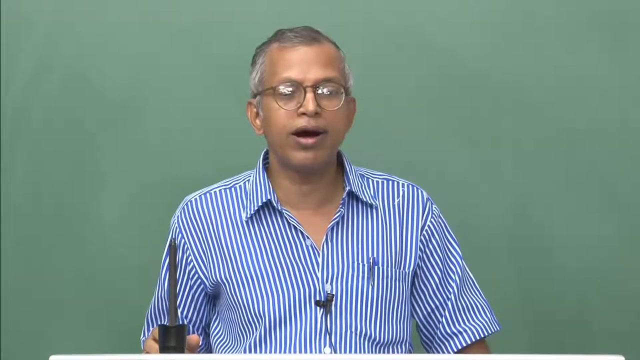 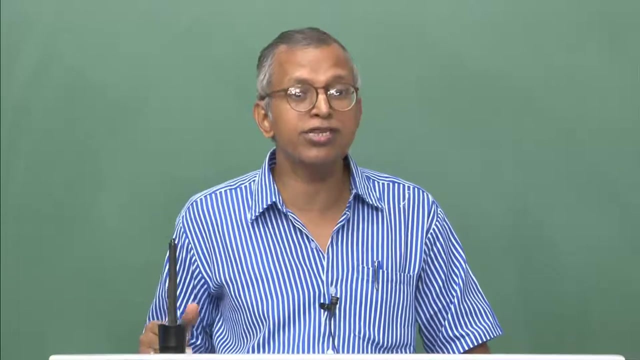 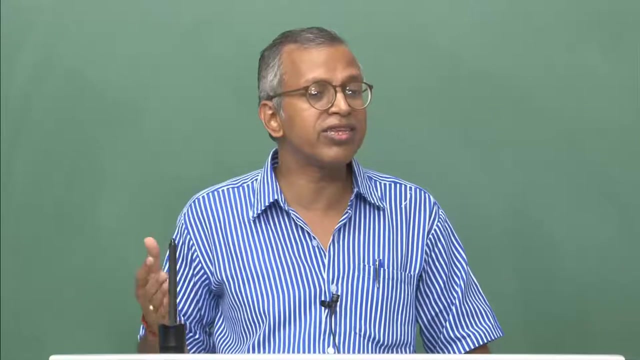 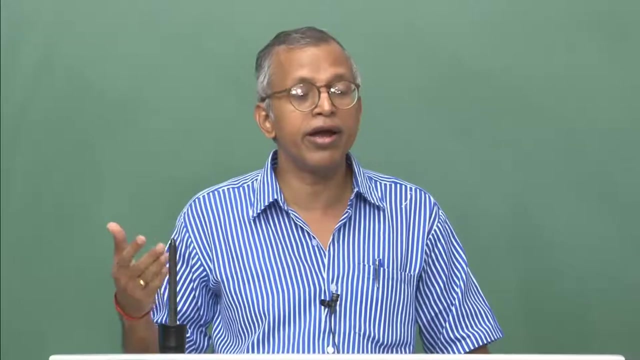 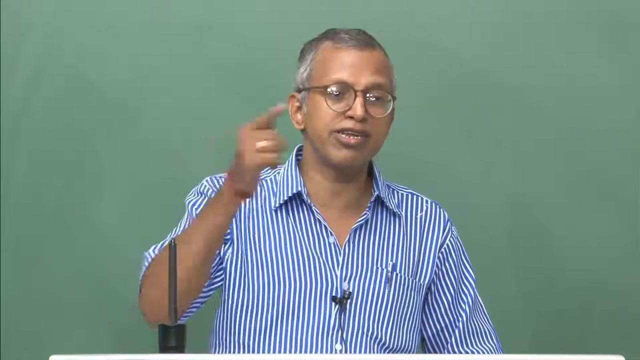 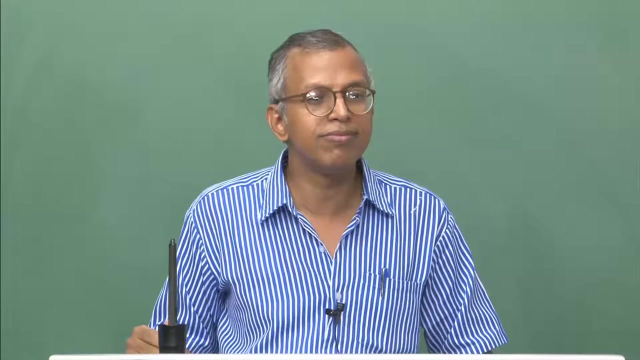 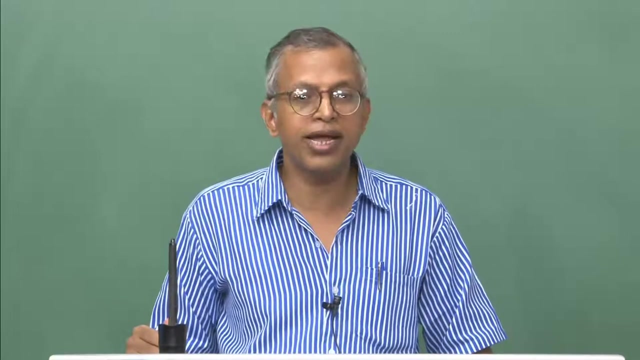 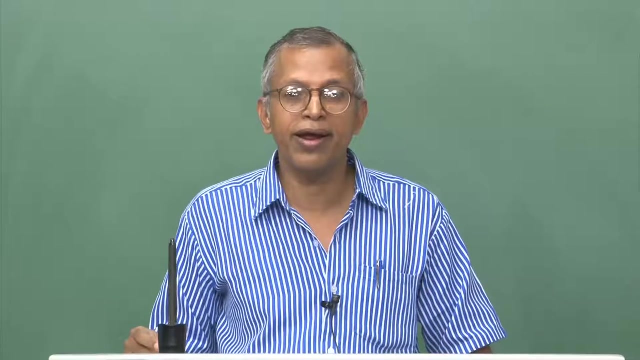 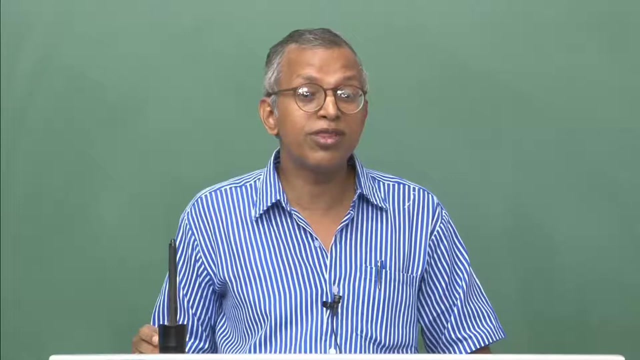 is basically, But we always try to reduce it. why it is so? Can anybody tell me The viscosity is a problem, but it can also be a solution some extent. Otherwise, if viscosity is not there, can I really make it to fly an aircraft? With this question we will move into several other. 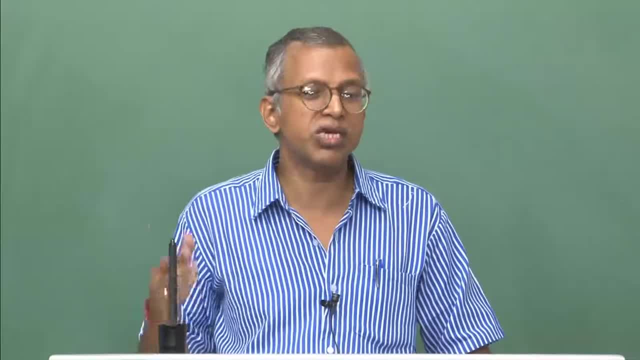 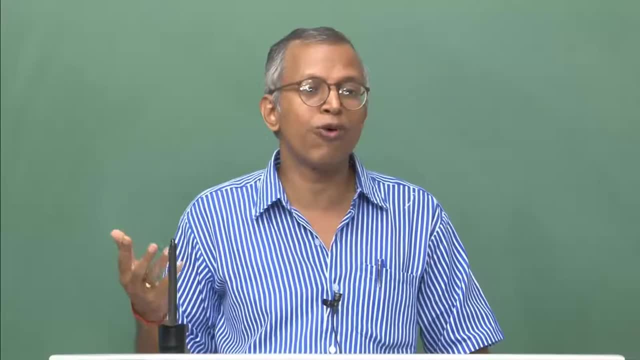 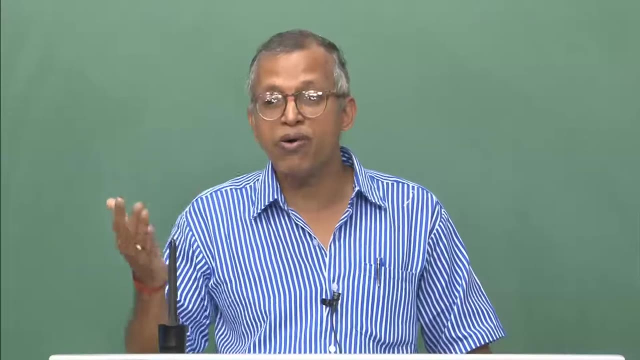 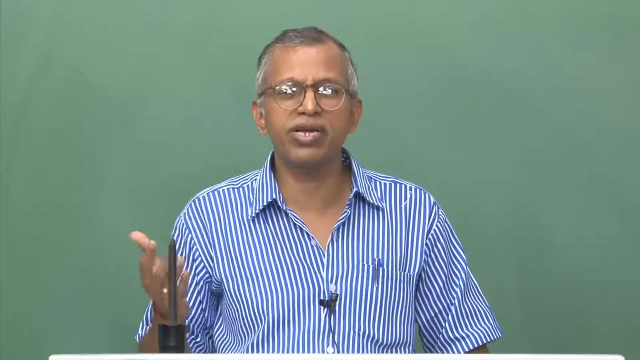 questions. To be very fair, there are three other aspects. What we discuss- Just to recall that we discuss about the effect of viscosity on the fluid. there are three effects: the進 2 effects- we talked about This diffuse fluid. 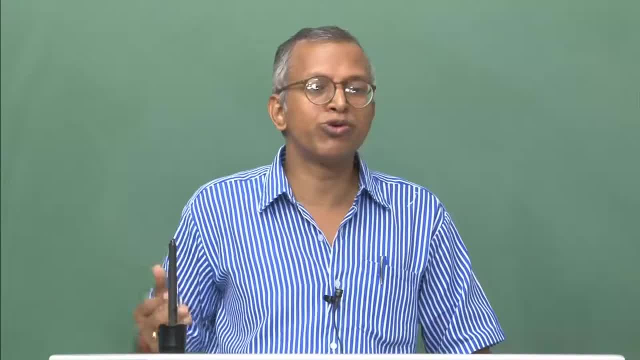 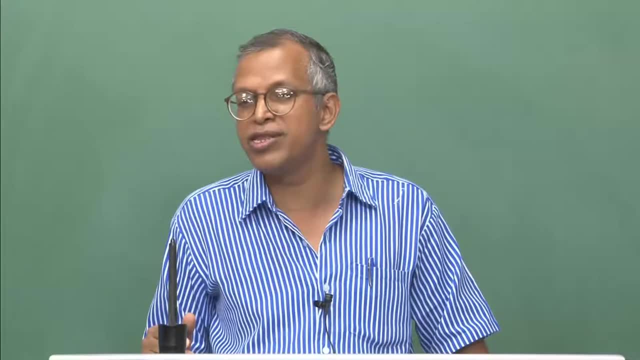 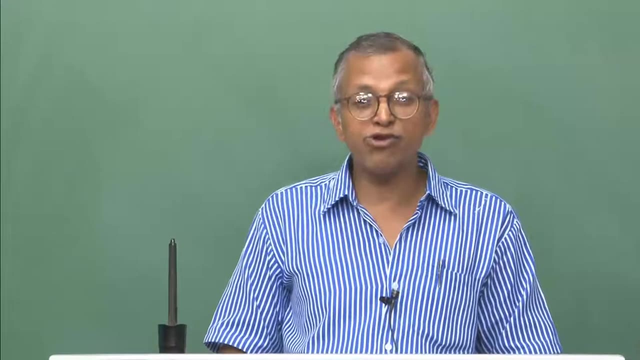 Now I am having one question to you. do you really understand what do you mean by steady and unsteady flow? I will ask this: we will try to answer this question today and I will check whether you have understood really what do you mean by steady and unsteady. but before, 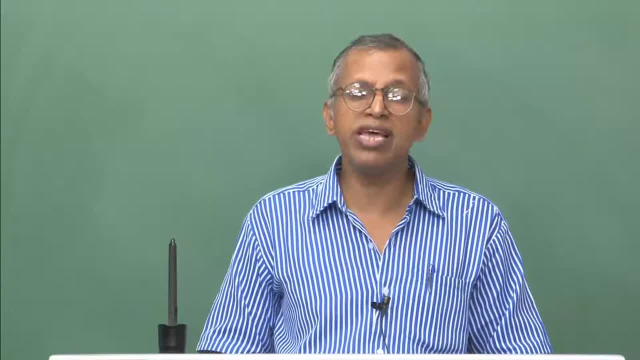 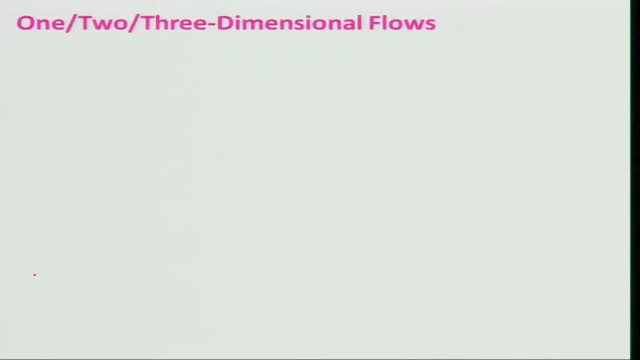 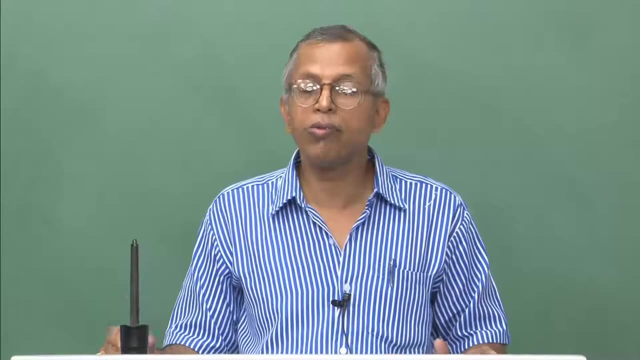 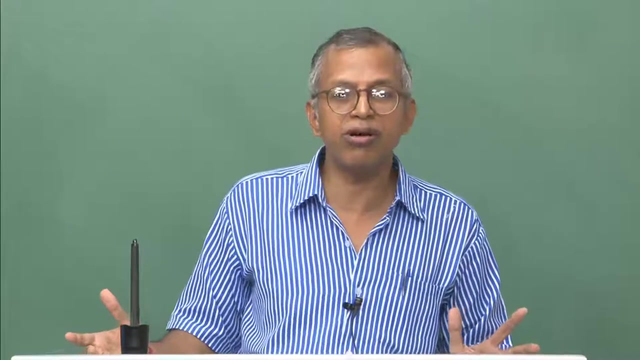 getting into that aspect. let us look at how many ways we can analyze the flow. We can think of the flow to be, you know, one dimensional flow, two dimensional flow and three dimensional flow. If you look at all, the natural flow will be three dimensional in nature. what 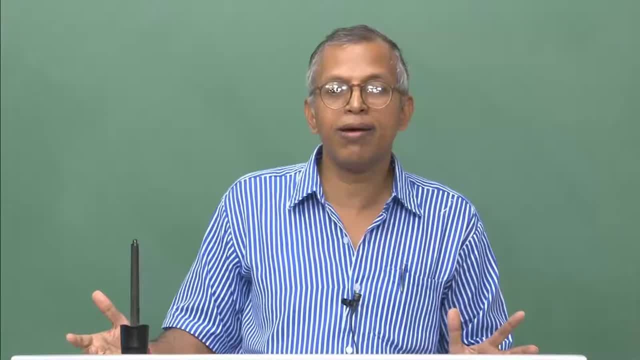 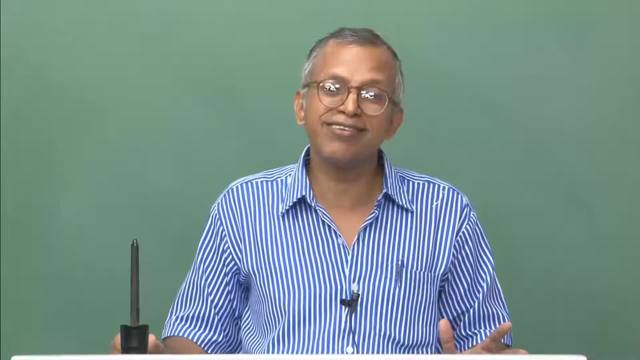 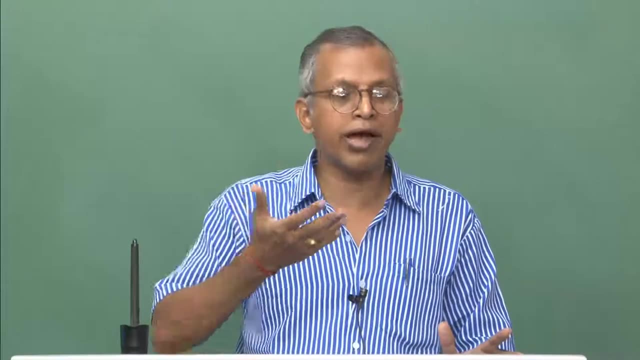 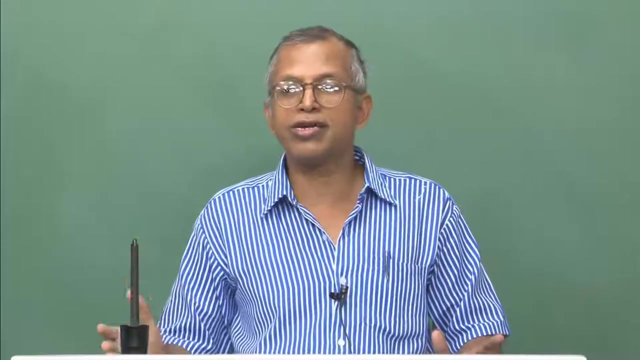 is the meaning All three dimension when you talk about dimension in a space, if I go where I will talk about dimension, When I take this room, I will be having certain dimensions, like I can say along one you know from a corner of a room. I will say that it is: one is x direction, other is y direction. 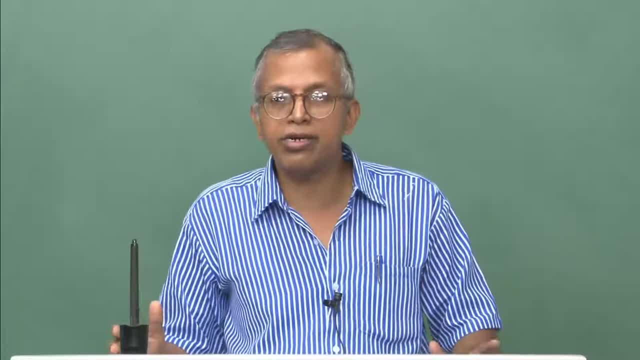 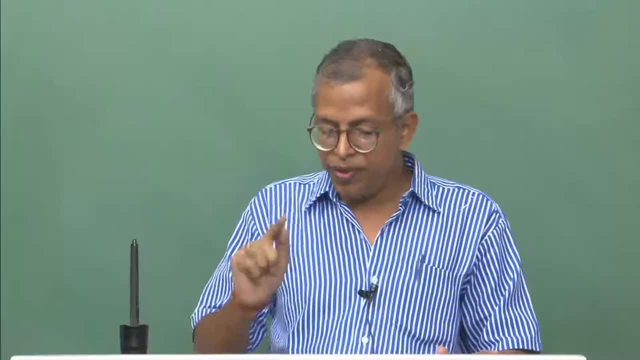 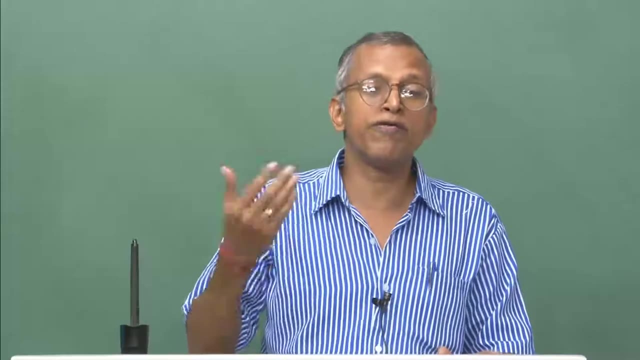 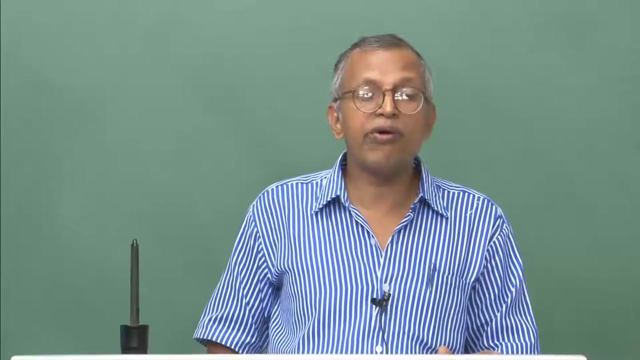 other is vertical. one is, you know, z direction or vertical direction, but in the space, what we will talk about- So that means the fluid, if you look at- is basically three dimensional in nature. However, for our own, you know, simplicity, or to analyze it, we always talk about a one. 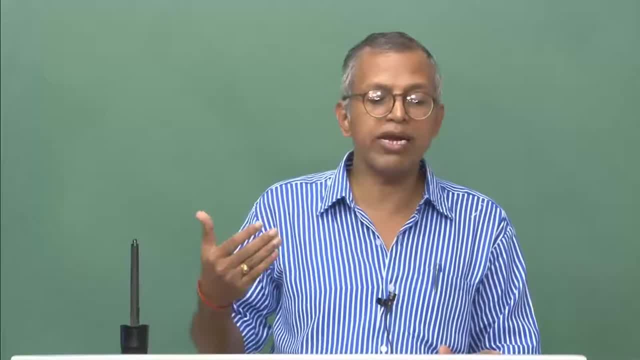 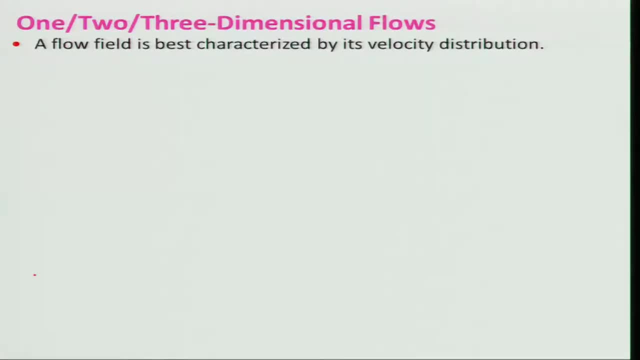 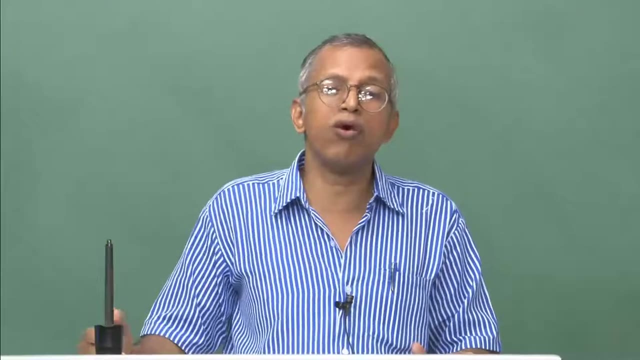 dimensional. What is that? One dimensional flow is one in which the flow field will be not remaining, you know, constant in other two dimension. only it will be varying in one direction. In other words, how we will characterize whether it is a one dimensional flow or two dimensional. 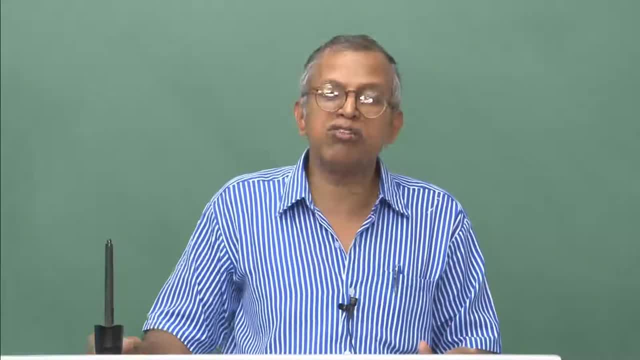 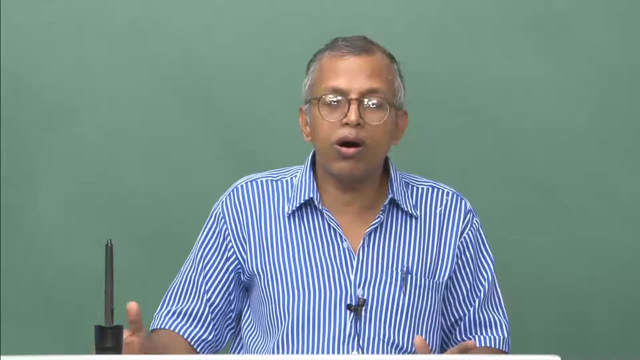 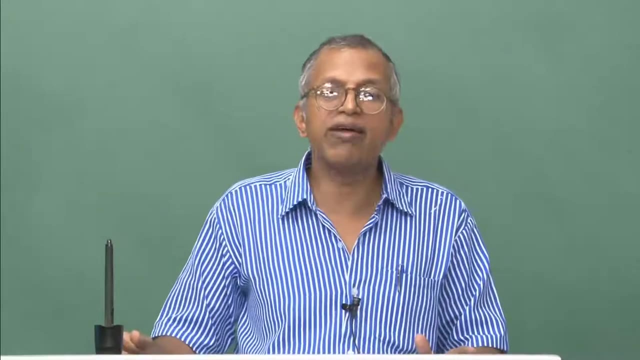 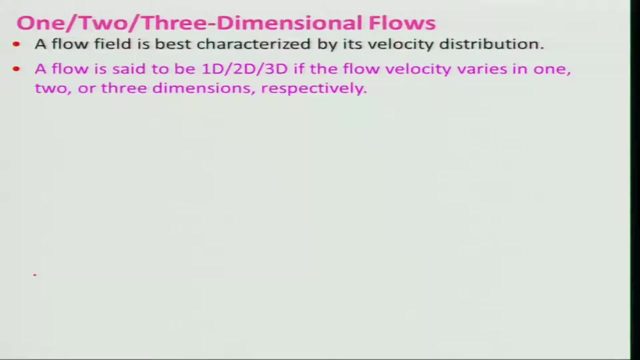 flow, We need to look at the velocity distribution. Okay, The velocity distribution generally, but you can talk about others. So, as temperature distribution and you know what you call the other properties like mass fraction, mole fractions in case of reacting flows, right, So a flow is said to be one dimensional, two dimensional, 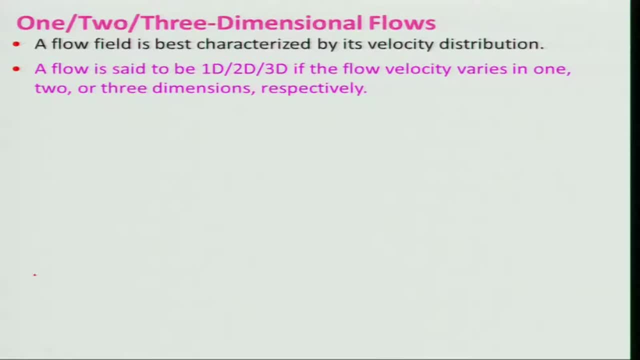 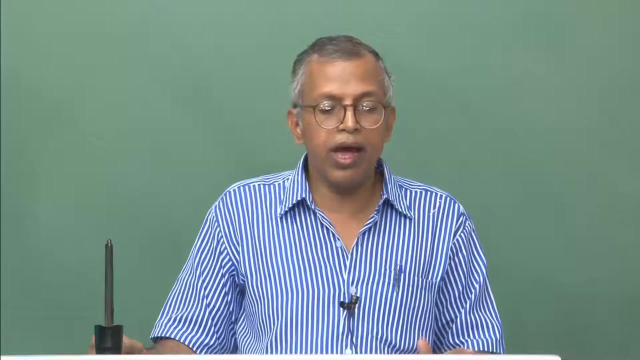 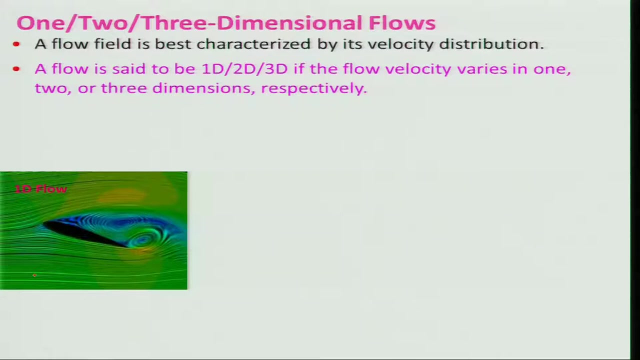 or three dimensional. if the fluid velocities varies in either in one dimensional or two or three dimensions respectively, right, then only we will be talking about it. and in case of a one-dimensional flow, which I have shown here, right, if you look at, this is a flow over. 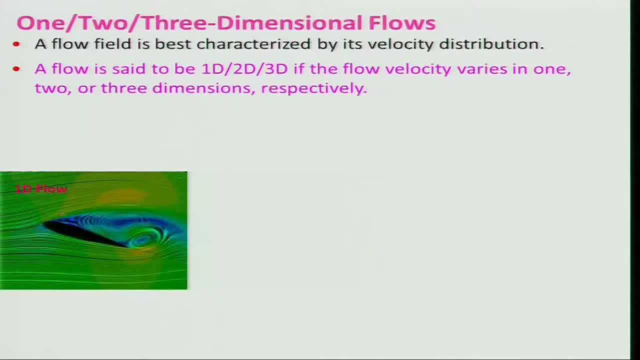 a and aerofoil. Where is the flow is one dimensional. can I say the flow is here is one dimensional. can I say here- some of you are saying yes, how it is possible? if I say this is my x direction, this is my y direction, Can I say: flow here is one dimensional? certainly. 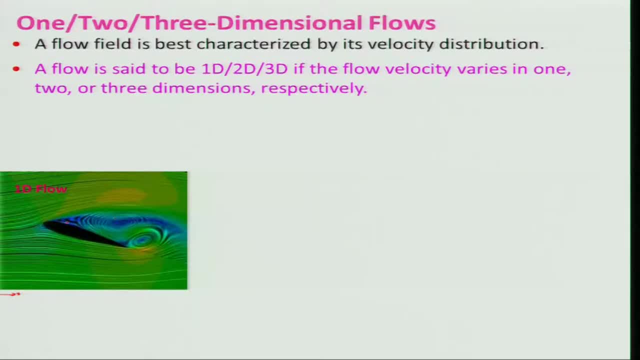 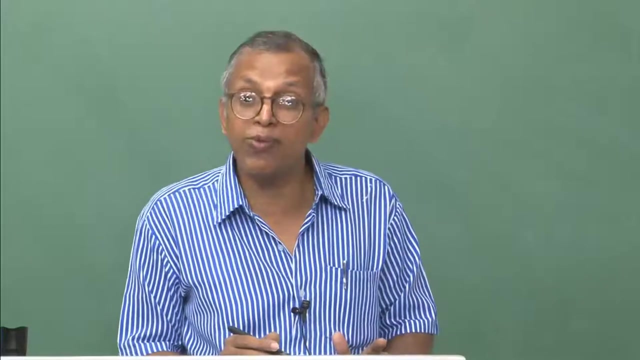 no, because there is a re circulation. flow is being separated at this point. similarly, I mean little away from the leading edge and in the trailing edge the flow is also re circulated. it separated and re circulating here, So I cannot call it as a one dimensional flow. 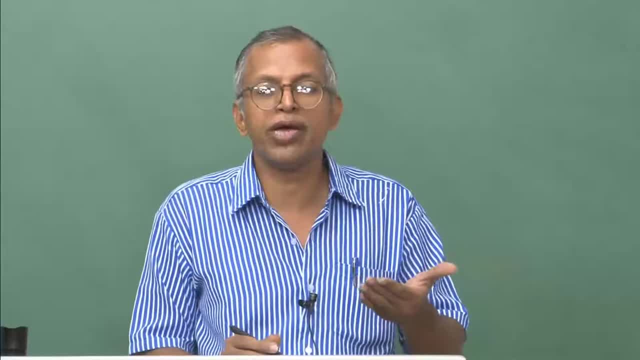 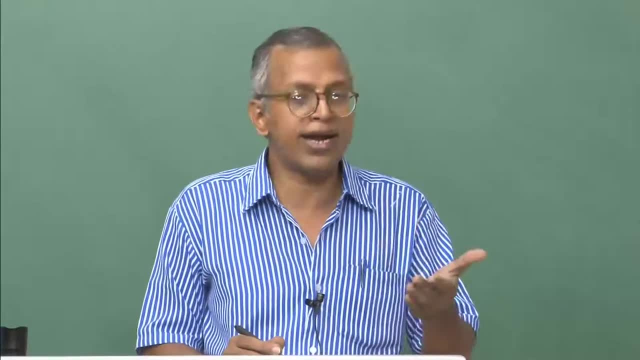 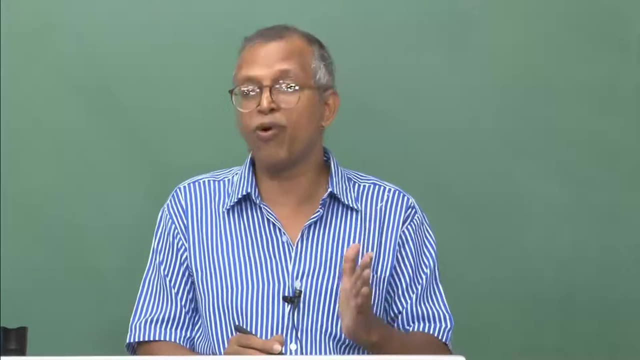 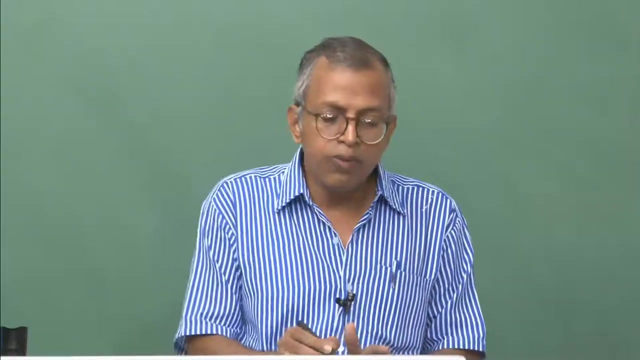 however, to create this kind of images, what you call flow visualization, there are various techniques. we use wind tunnel or a water tunnel, which is where you can have a control over the fluid flow velocity And also its distribution. in this case, people have assume the flow to be one one dimensional. 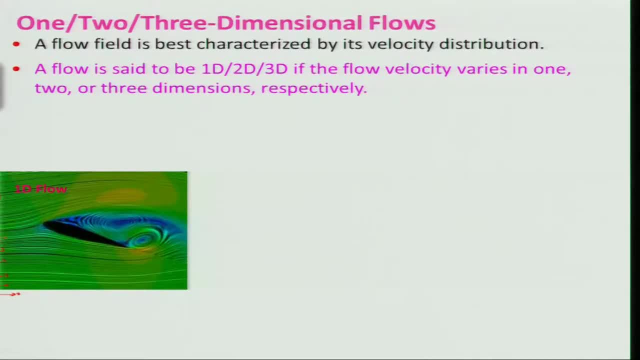 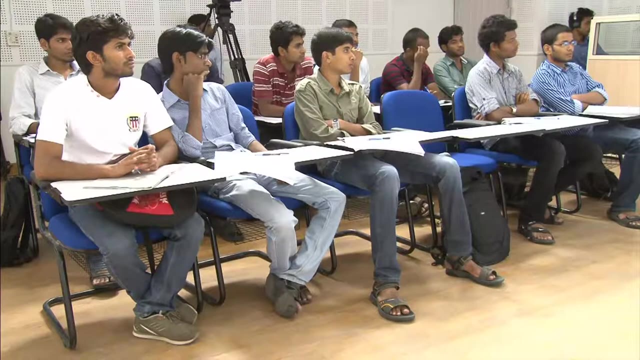 here. that means this is the uniform velocity. what you can see is it? you can observe this. what are these lines? if you look at, these are the some lines. what are these lines? these are stream lines. are you sure it is stream line? What do you mean by stream line? 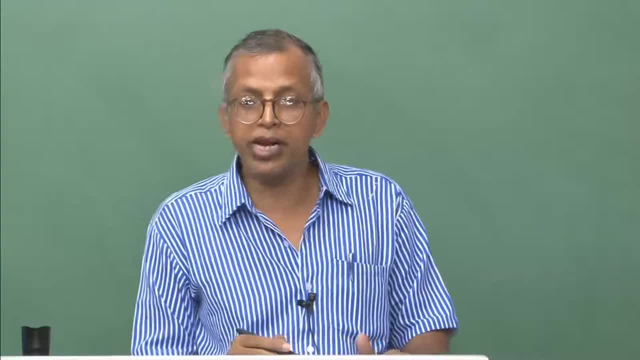 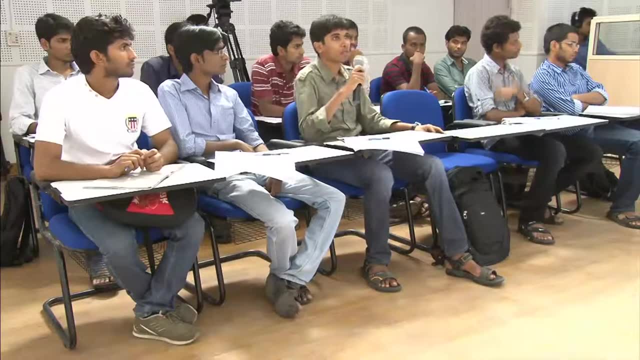 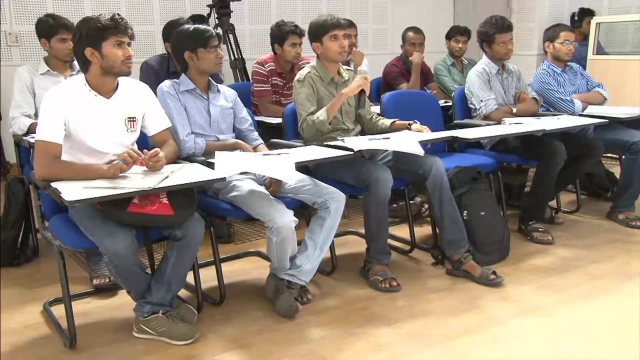 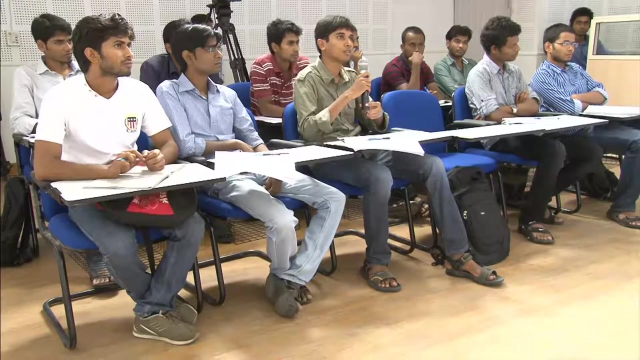 Can anybody tell me, please, what do you mean by stream line? Path trace by the fluid particles in a flow is known as stream line. are you sure what you are saying? Stream line, that means both are same. what you are saying? am I right or wrong? can anybody? 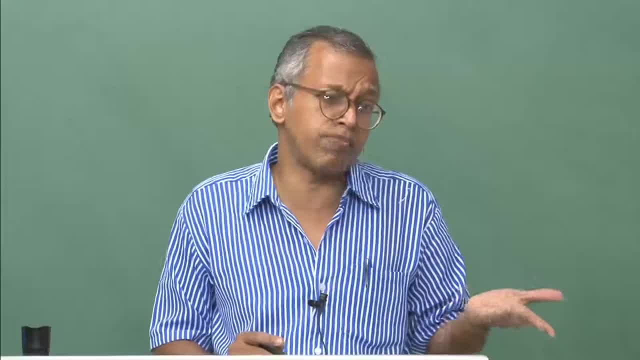 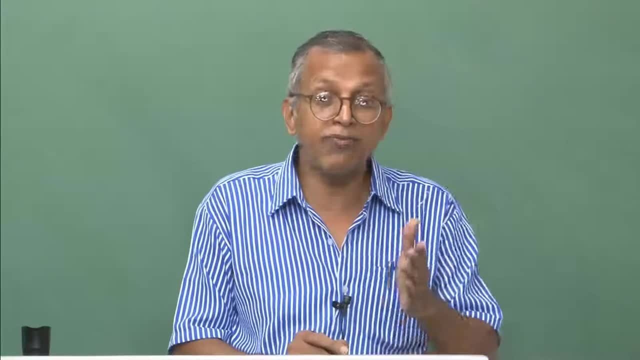 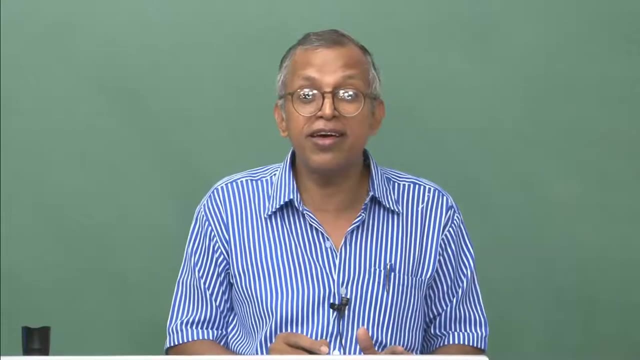 tell me What is the difference between these two? or both are same in this photograph. is it stream line or path line? because first definition, what you told it is a path line. the second definition, what you says it is a stream line. in this case, what kind of lines we are having? 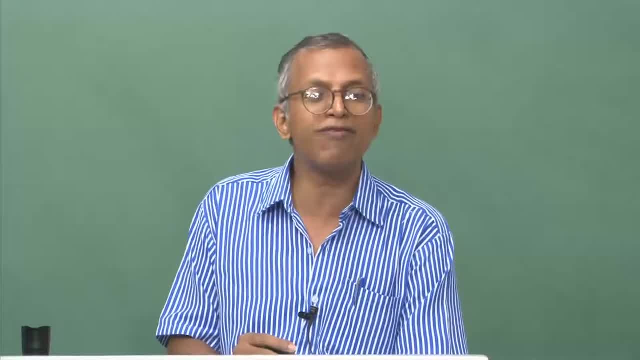 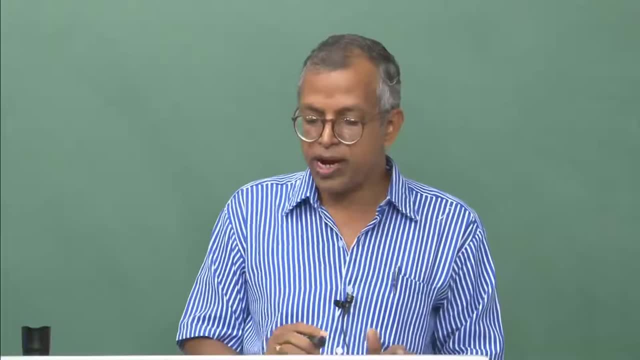 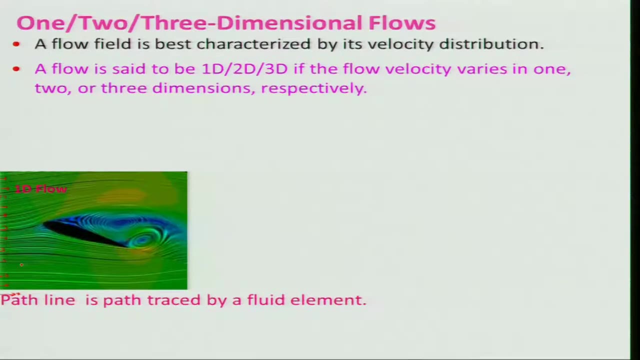 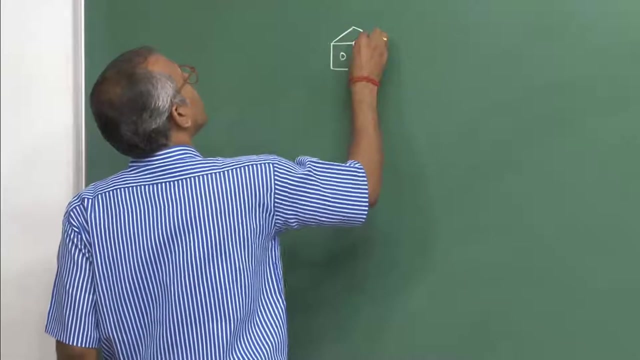 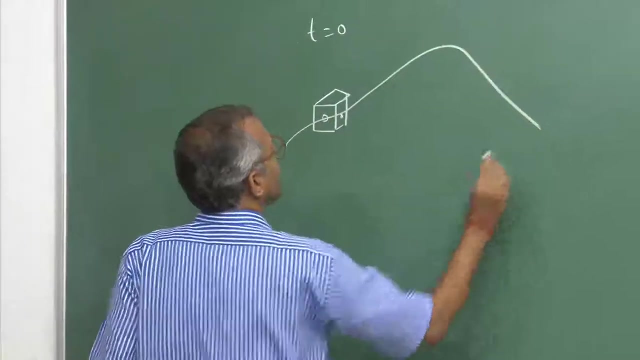 because these lines are very important for visualizing the flow, Right? So, coming back to this, This path line is basically path trace by a fluid element, right? what do you mean by this? suppose I will take a fluid element here, right, and at time t is equal to 0. let us say: 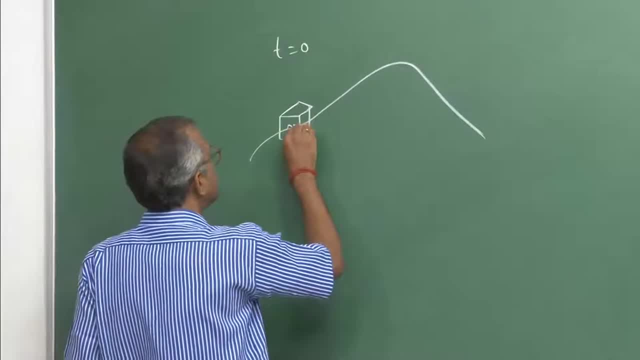 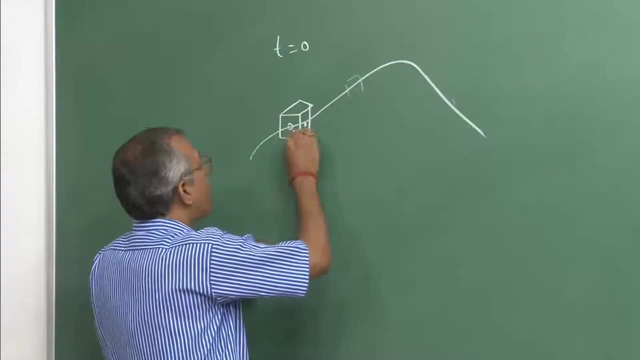 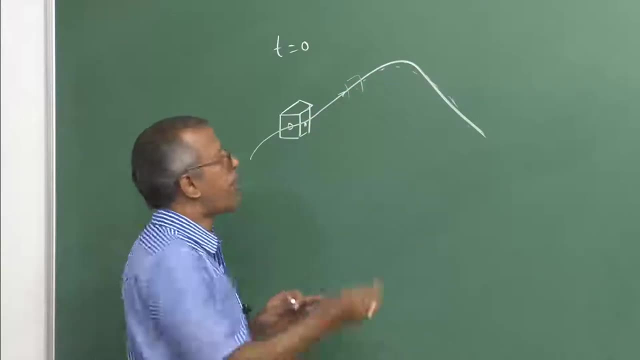 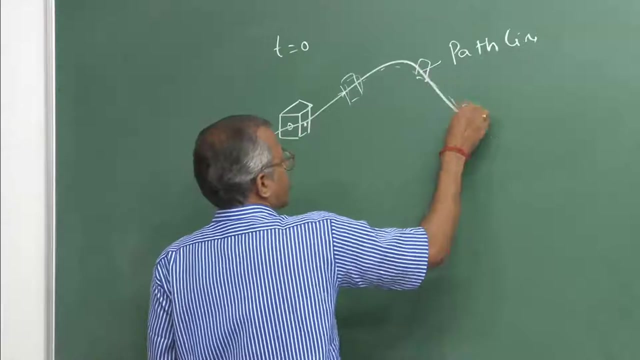 it is moves like this. right, that means at, fluid is here And at certain time it will be going over there and other things. right, that means the time trace by this fluid element along this path will tell me the path line. right, It is here, it will go over there. it will go over there. it will go over there, right that? 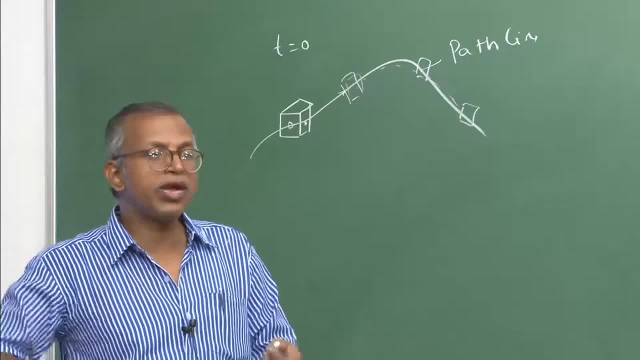 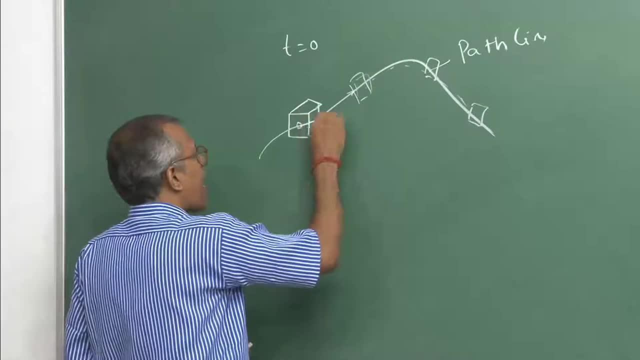 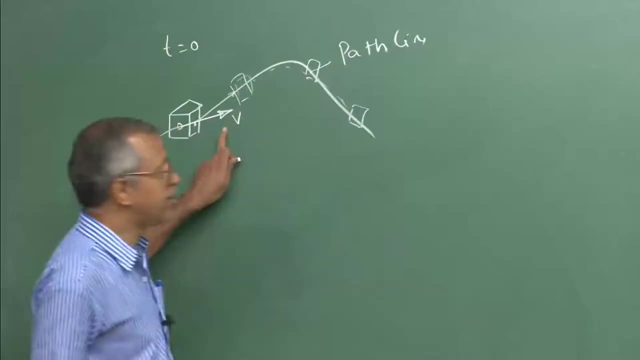 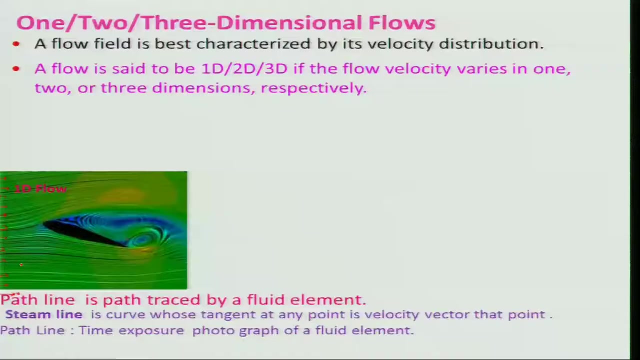 is known as path line, right, but then when we will call it as a stream line, That means it is when it is fluid. fluid is having a velocity, right, yes or no? that means this is the vector. as you told, that stream line will be basically a curve whose tangent 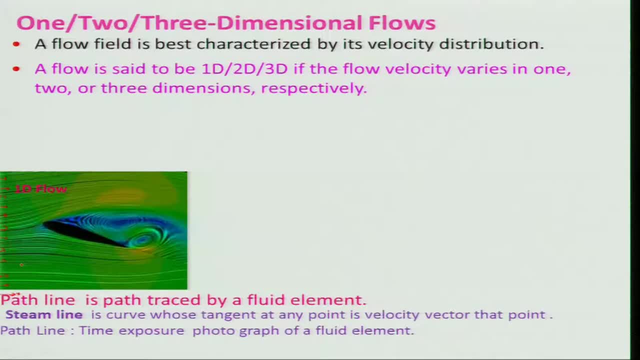 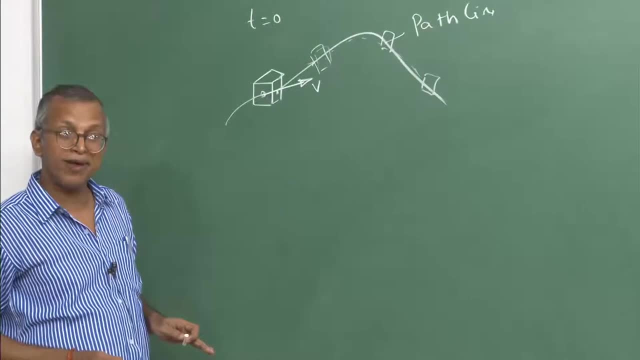 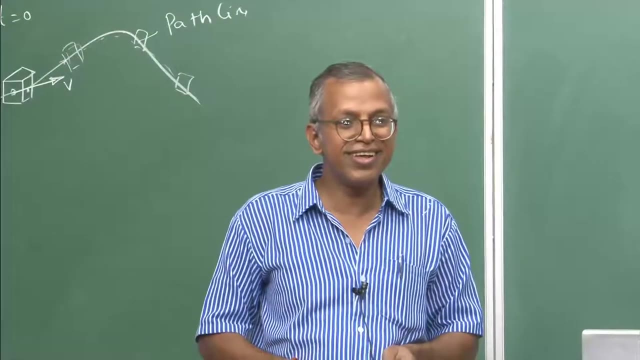 at any point? is velocity vector at that point right? Will you call it as a stream line Then? Yes, Because I am showing the same thing, like you know, in the same line. can I call it as, Sir? uniform flow is stream as a same flow. 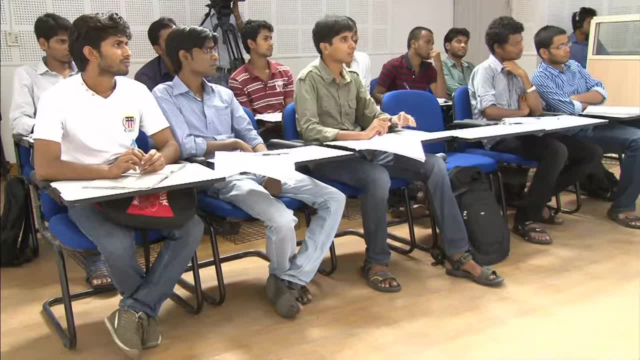 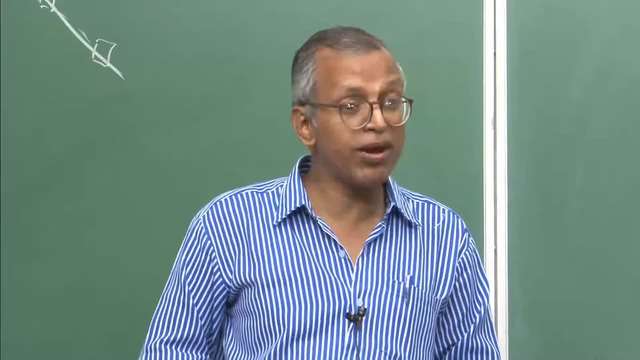 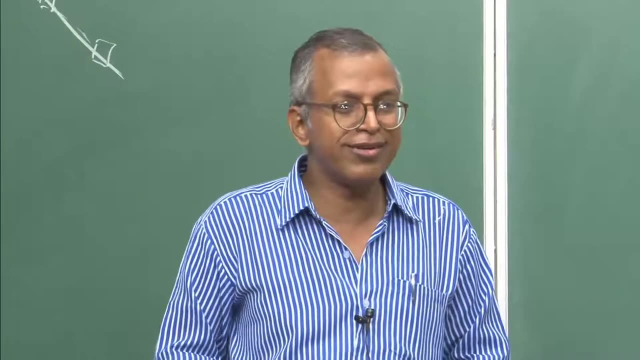 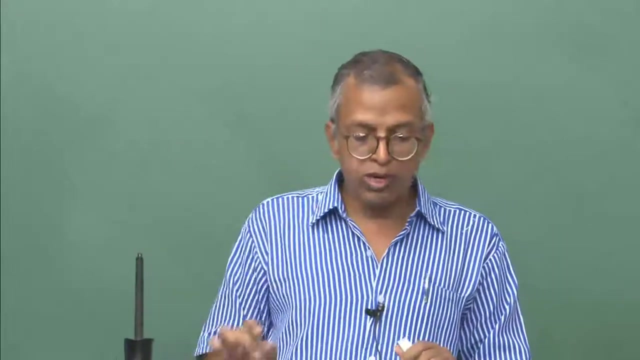 Uniform flow For steady flow. I think the second answer- what is given by him is the right- is a steady flow. that means what is the meaning? how I will get a path line whenever I am conducting experiment, How That means that will be time exposure of a photograph or time exposure photograph of 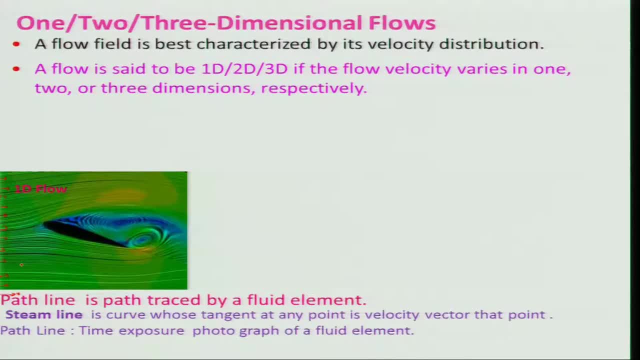 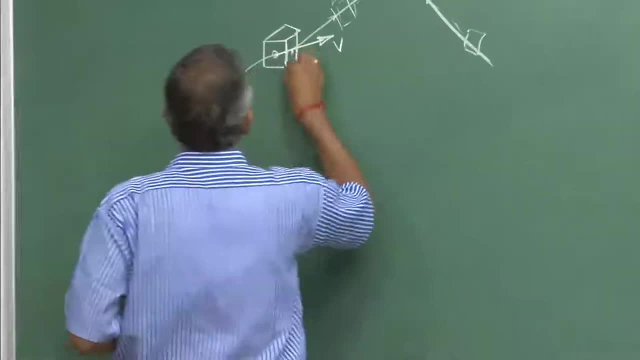 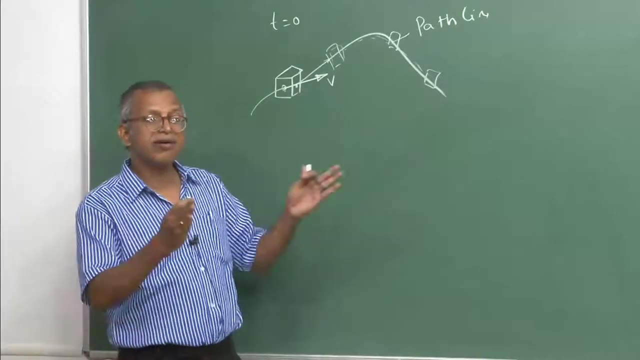 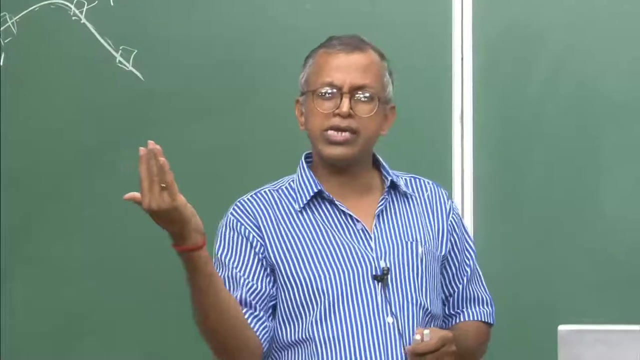 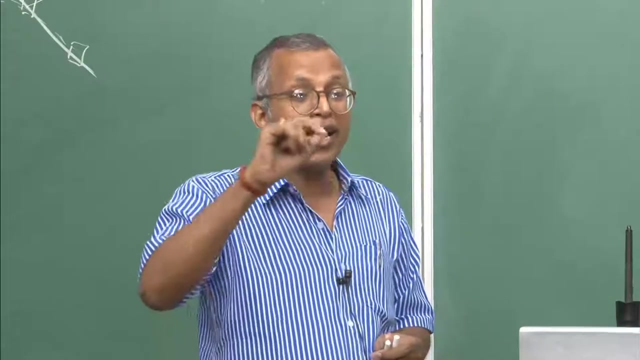 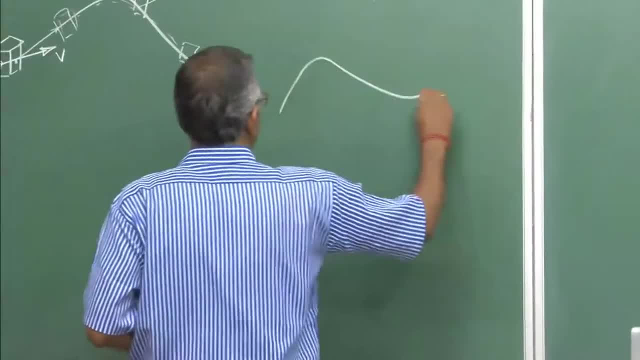 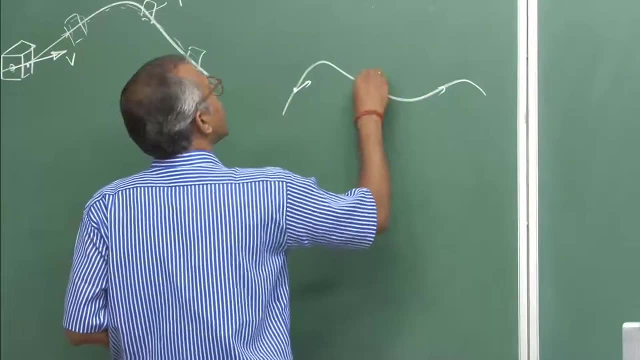 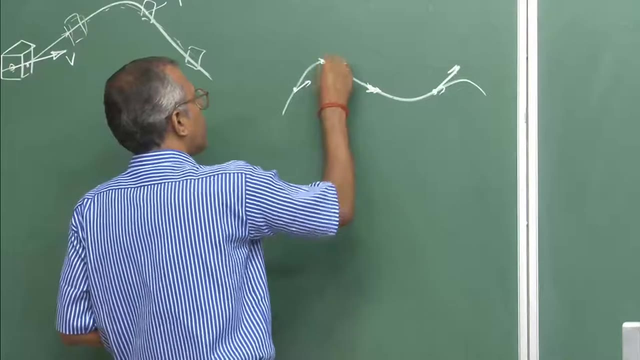 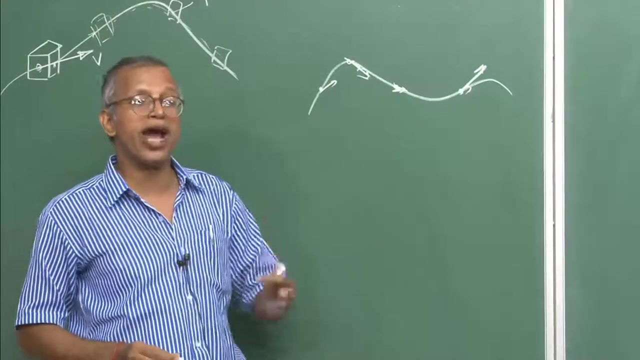 what is the velocity vector? for example, let us say this is the my, you know, flow is taking place here. I can say that this velocity is here and this velocity here may be. this velocity is there at that point right. That means this picture I have taken at one frame of time may be at instant right. and what? 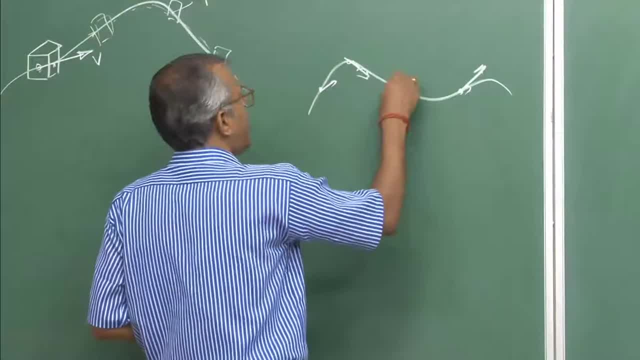 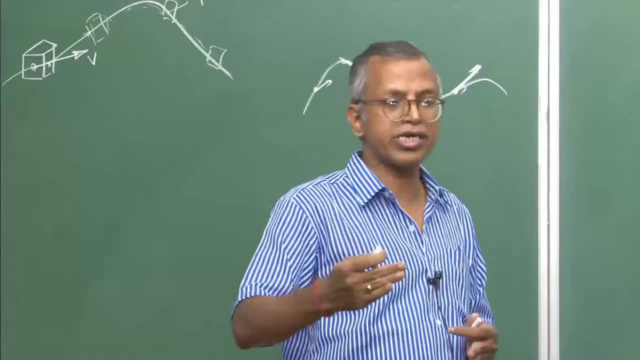 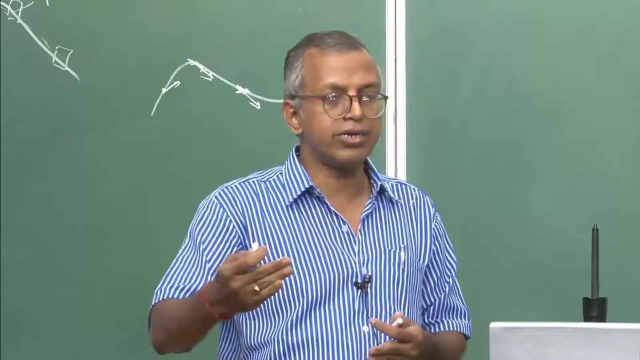 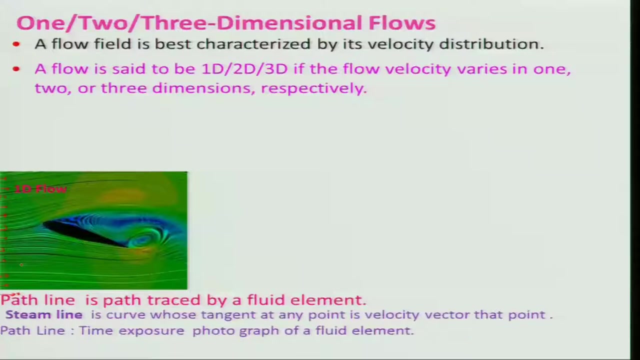 I need to do. the fluid element will be there, and then it is some. you know, I am just taking a vector looking at velocity. velocity is the vector quantity, it is having magnitude, it is having a direction Right. So then I call it as and I can obtain, if I will be getting what you call a single frame. 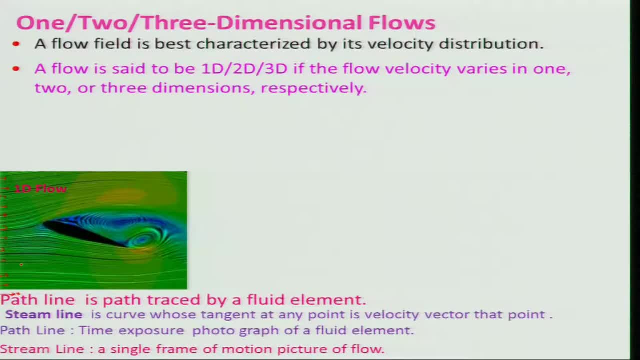 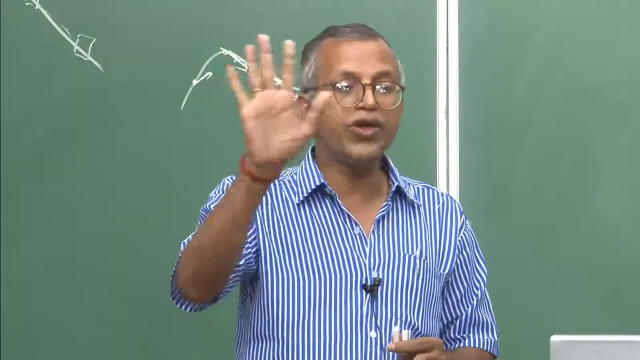 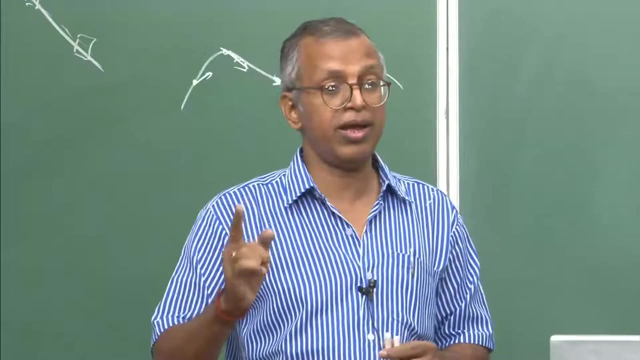 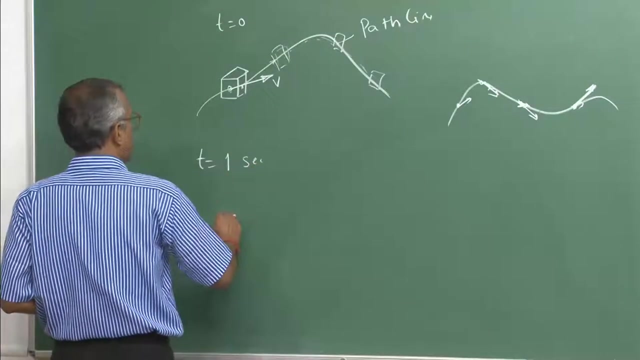 of a motion picture of the flow, right? So you know I can take a video at one instant of time, right, I will get full what you call view of the entire domain on which I have focus, right, that is basically a stream line, But when I take this time, t is equal to, let us say, one second, this image. you know this. 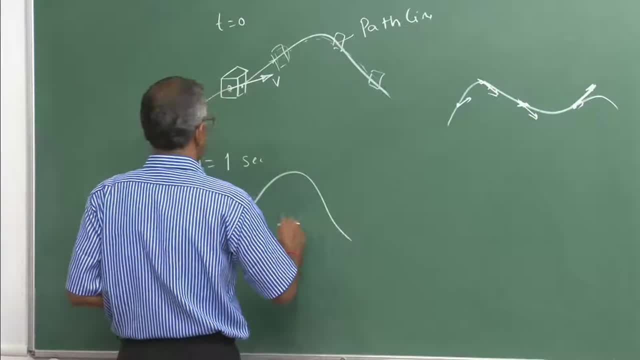 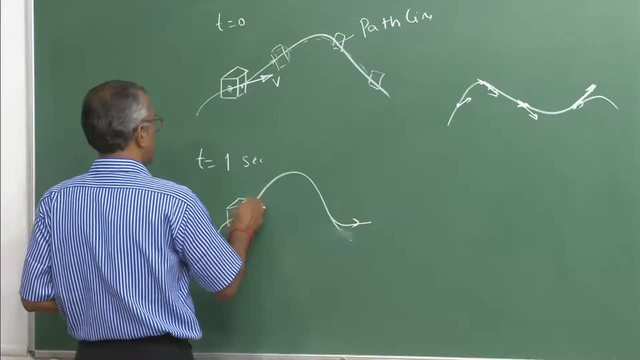 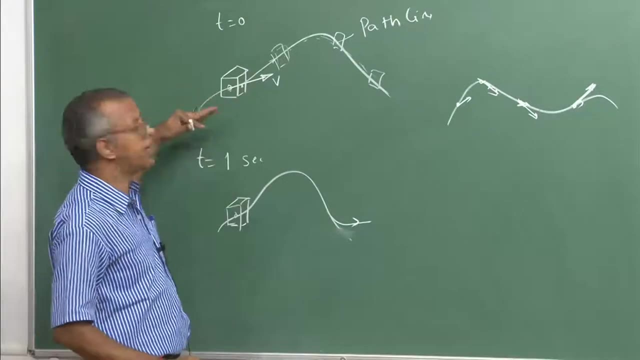 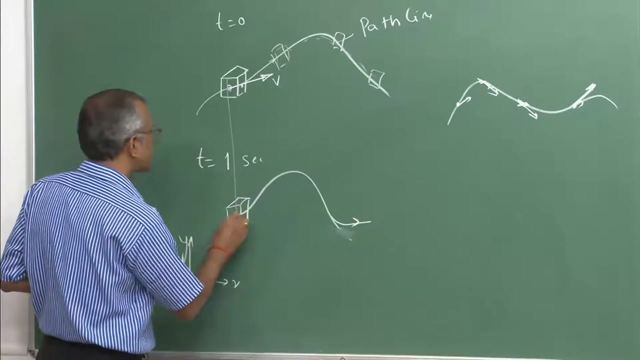 path may take a different path, kind of things. this can take a different path, right? So then this will be what you call unsteady phenomena, right? that means I am the at the same location, same. If I take this is x and this is y, I am having certain distance here. the distance is almost. 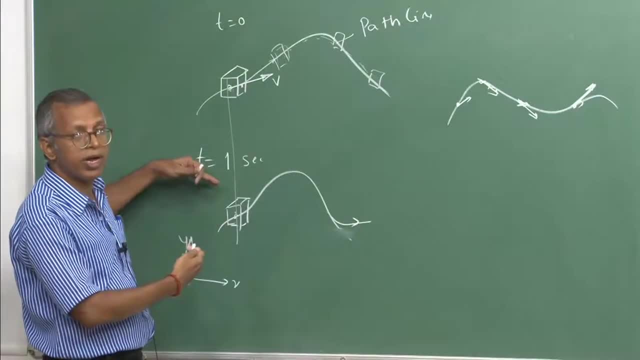 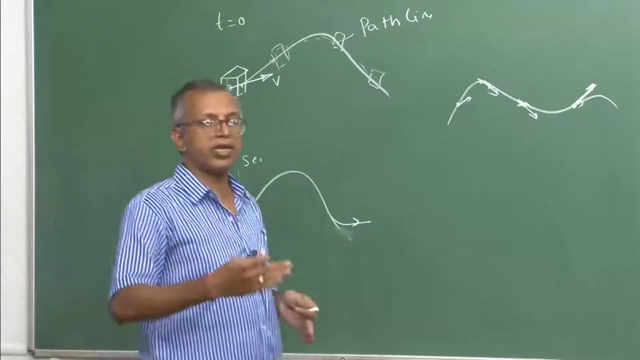 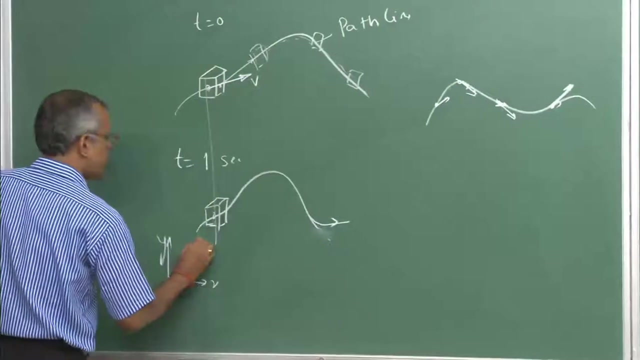 same, but I am plotting at different time. step right upon this reference o you know, it is having same dimension. let us say 3 meter from one side and another point is 4 meter. x is equal to 3 meter, y is equal to 4 meter. at this point I am measuring a, you know point. 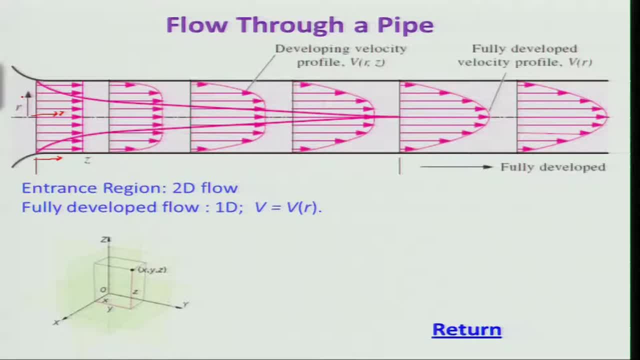 your z direction. this is your r direction, right. So this is a what you call a another coordinate system. what we will talk about it, that is known as r theta z coordinate, or the cylindrical coordinates, right In this case, what we are considering in the z direction. keep in mind that in this figure, 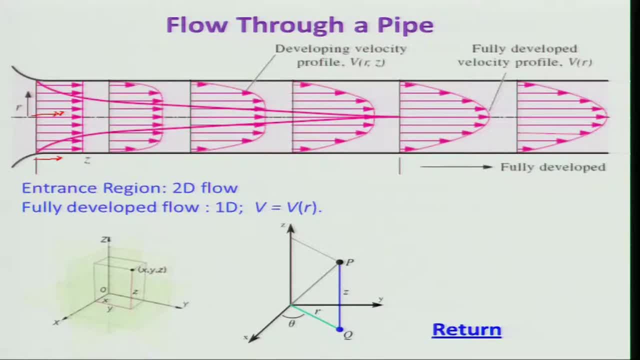 z direction in this is a from left hand side to right hand side and this is a r direction, right, and theta direction is here, it is moving. So you take a this thing and move around a theta, then you will get a pipe, kind of things. 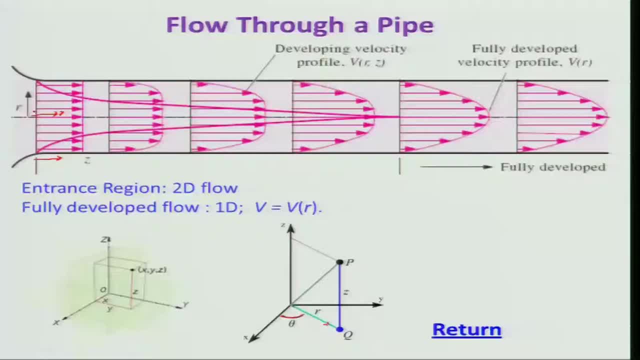 right. So here we are considering basically a, z and r right. that means velocity is changing along the z direction. if you look at started with uniform velocity, what happens to this velocity profile? it is different that the beginning of the uniform velocity profile. it goes on changing. 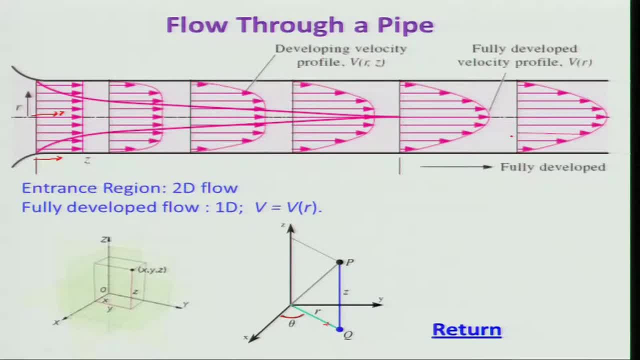 Right along the z direction- yes or no right? and also it is changing a particularly here along the radial direction: yes or no right? in this point it is all changing along with this, whereas at the entrance there is no change in velocity along the radial direction. 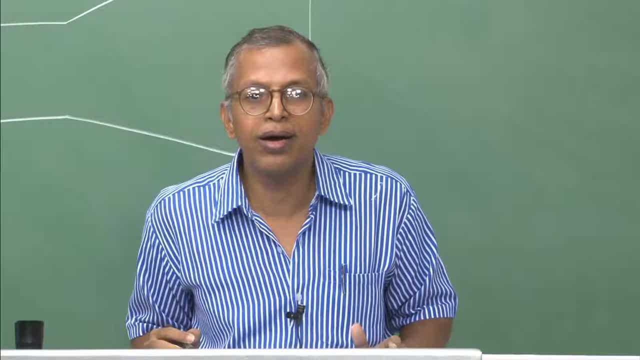 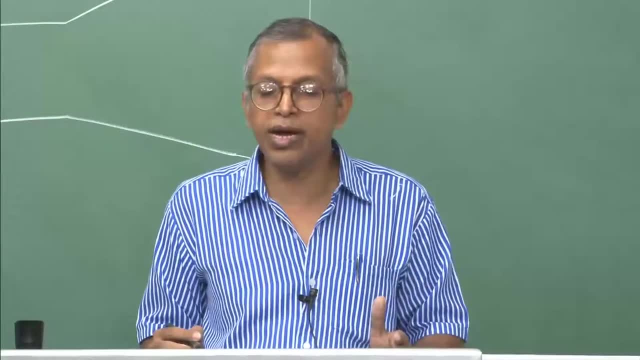 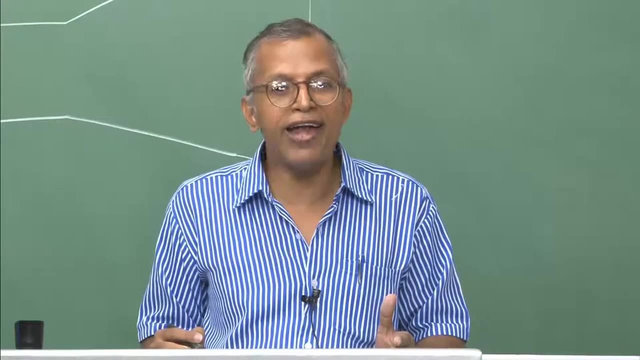 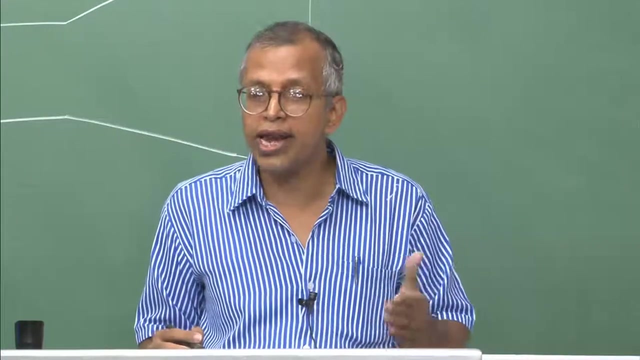 but what happens to theta? Is it changing or not? in this figure what I have drawn, or we can assume here that it is only the velocity, particularly it changing along with the r and z direction. that means it is a two dimensional flow. can you call it two dimensional flow or I will have to. 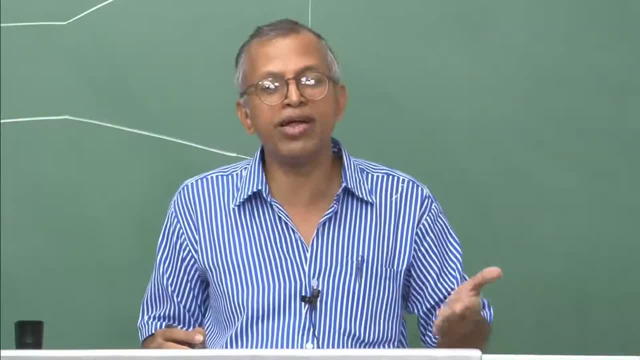 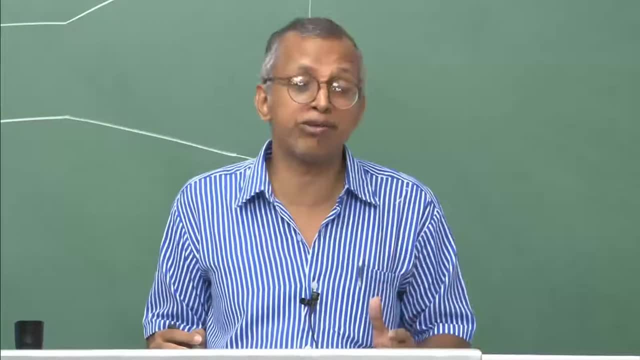 tell two dimensional axis, symmetric flow or, in simpler axis, symmetric, you know, Flow kind of thing, because along the theta direction I am saying it is symmetric So I need not to consider it is uniform, that right. So you need to understand what is. 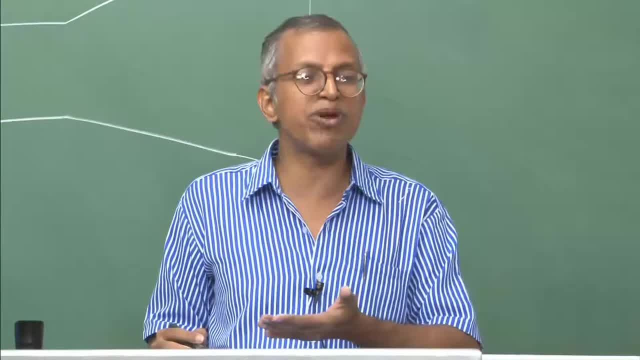 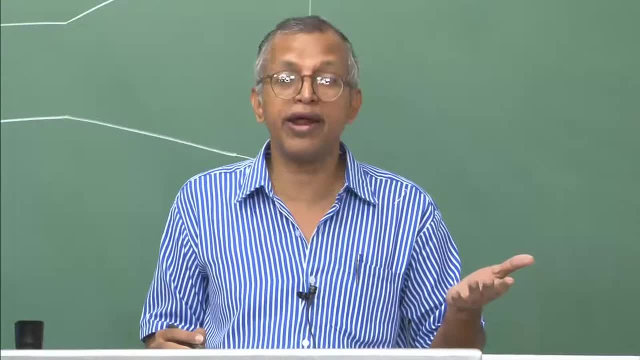 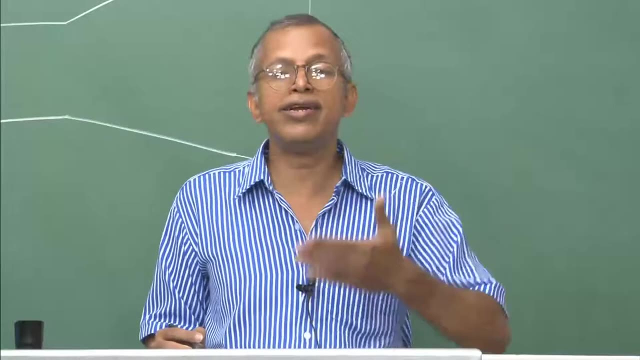 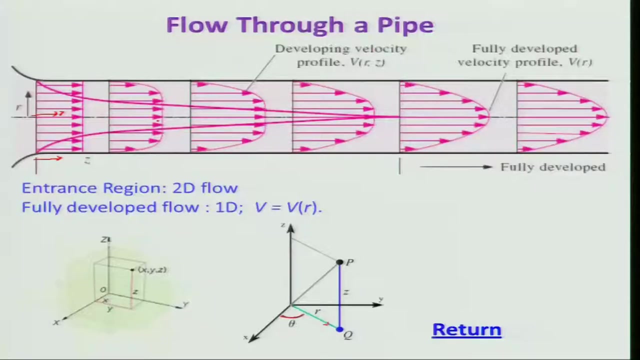 the difference between pure two dimensional flow and axis symmetric flow. it is very important because we will be dealing with axis symmetric flow most of the times, right, because all our aerospace ducts and other thing will be cylindrical in nature, So cylindrical coordinate system is more natural to be used. and what happens to the? 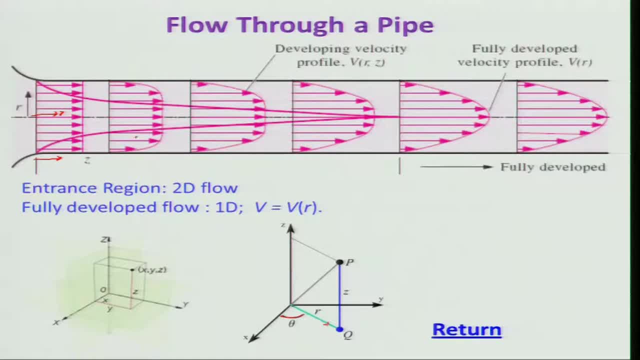 velocity you look at here like it becomes, you know, changing, and when you go to here there is a increase in this and then it becomes also become changing. and what is happening here, the velocity profile, And in this, what is happening? if I compare this two velocity profile here and here, what 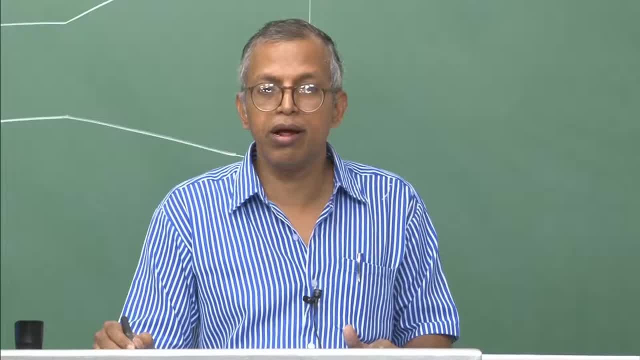 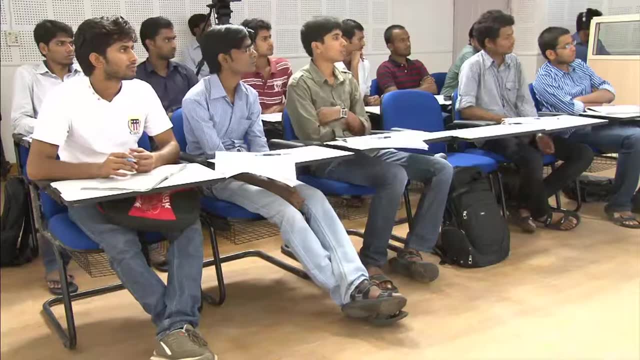 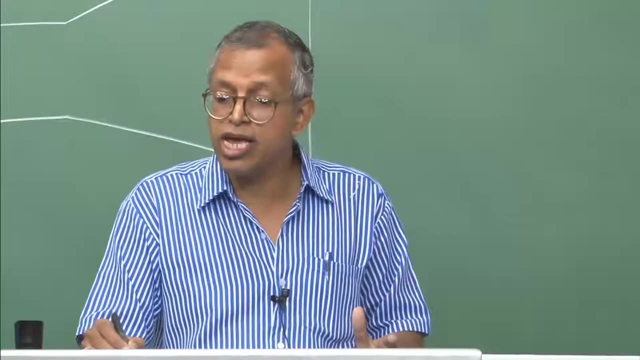 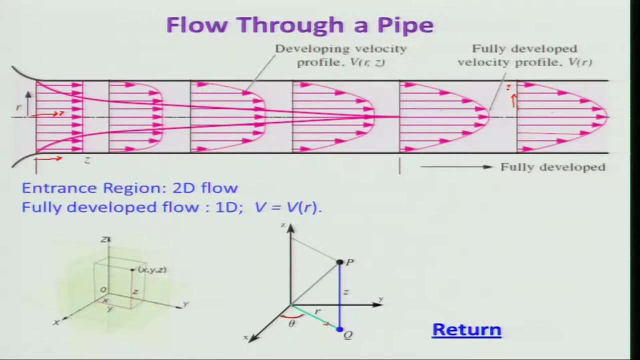 is happening. can anybody tell me 1 d flow how you are saying it? It is not changing along with the z direction. However, the change in the r direction- right, this is r direction. it is changing. therefore we can call it as a one dimensional flow, but why it is happening? 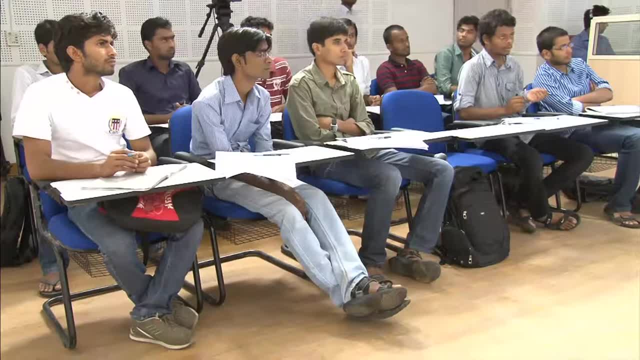 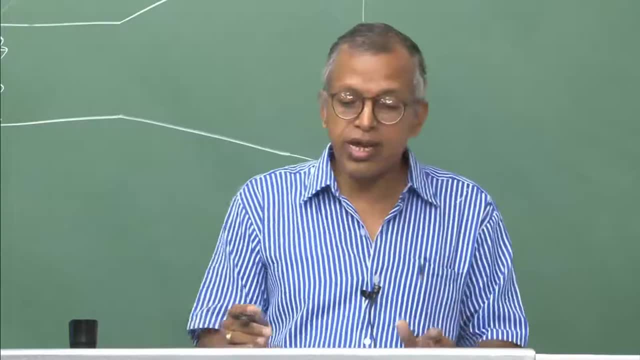 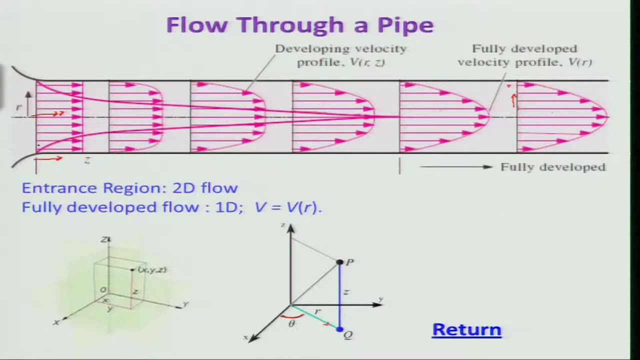 why means why it is fully developed. you call how it is happening. It is because the this line, what I have shown here, indicates the boundary layer which is grown from the inlet of the pipe. it merges after that. there is nothing really happening with the boundary layer because 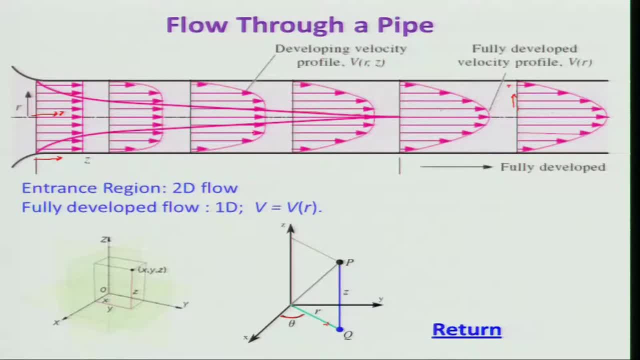 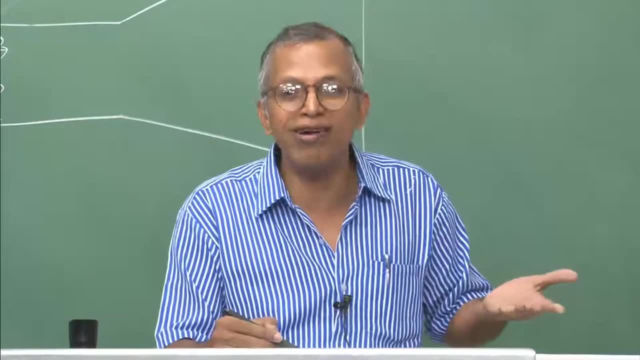 boundary layer, two boundary layer: upper boundary layer, lower boundary layer. of course I cannot say upper and lower, but it is a pipe, right, if it is channel, I can say upper and lower boundary layer. in a pipe, what I will say upper and lower, it is along with the theta, you know. 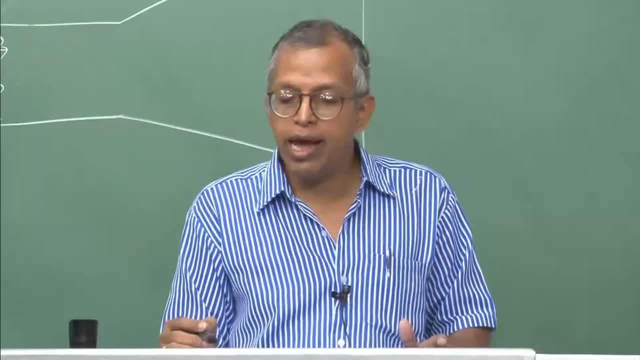 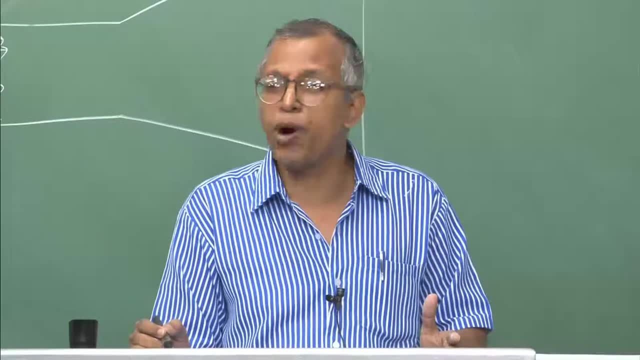 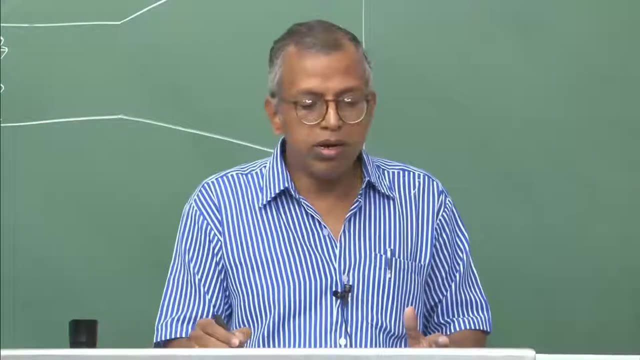 like whole circumference is being merged, And when it is merged that is known as fully developed flow. and for that you know, equations are there, Poiseuille, equations you can solve, that you might have exposed in your fluid mechanics course. But now what is happening to this velocity in this zone, what I call these velocities? 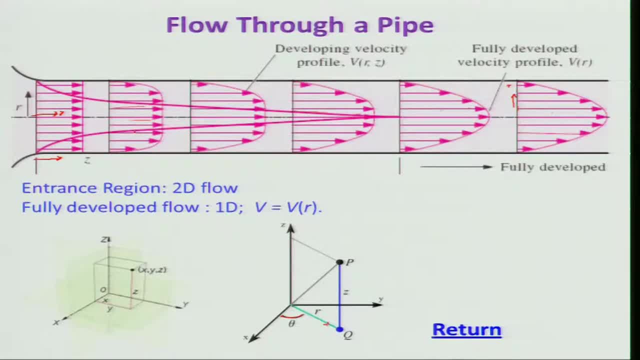 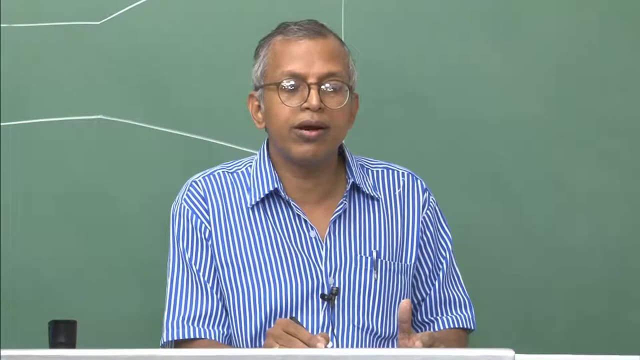 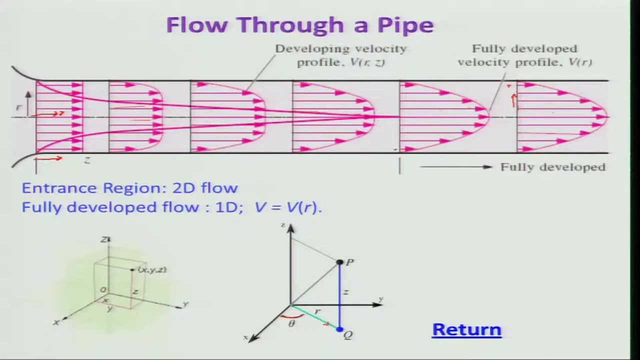 and these velocities and these velocities, what it is. this is known as the core region in your jet flow. You must be knowing we will be discussing little later on jet flow right where the core region is, there, what you call it as a core region. I will leave that question Now. question let us get into at what distance. 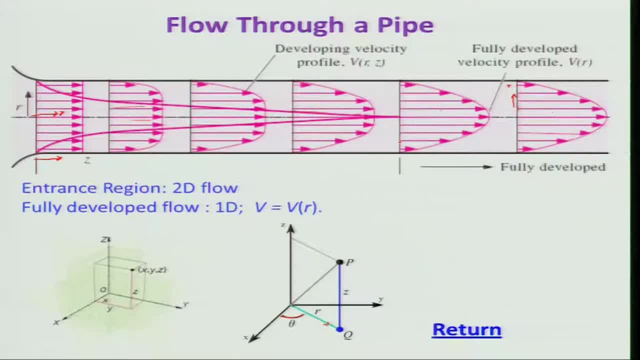 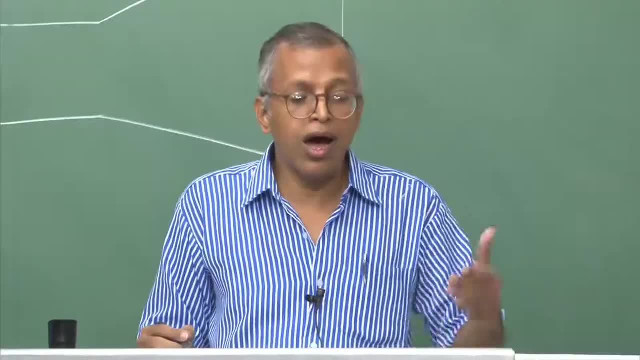 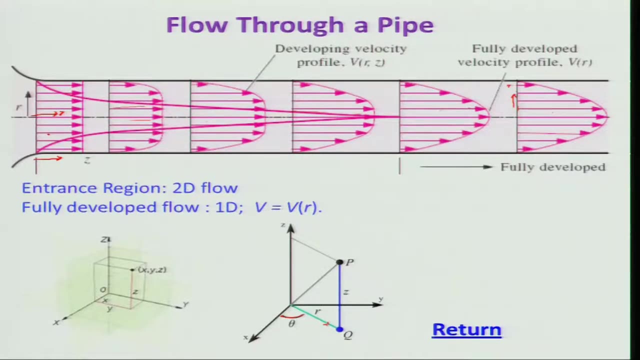 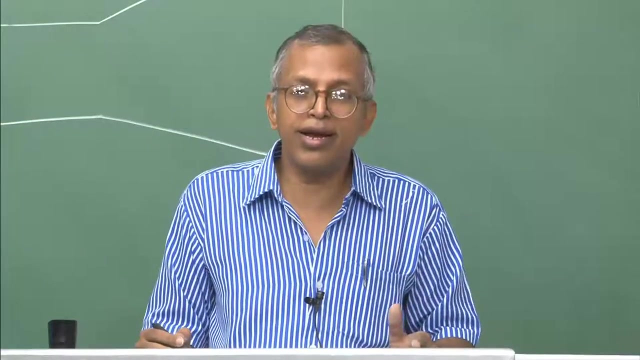 I should get a fully developed flow. will it be dependent on what? will it? will it be dependent on inlet velocity profile? will it dependent on the how this flow is entering? basically, I am saying the same thing in a different word. Then what else? will it be dependent on laminar or turbulent nature of the flow at the inlet? 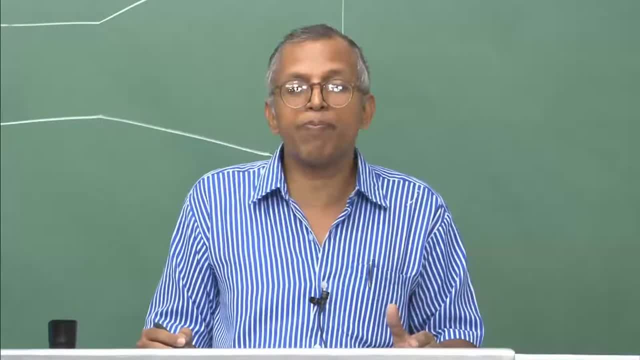 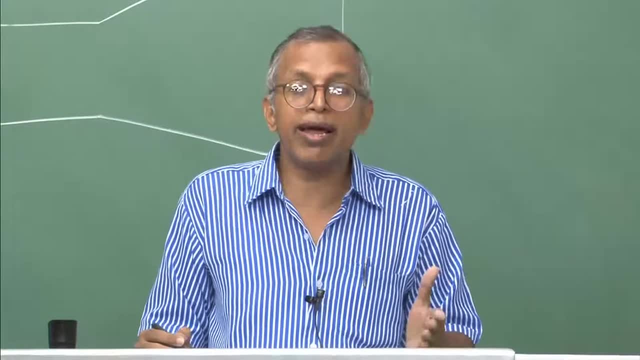 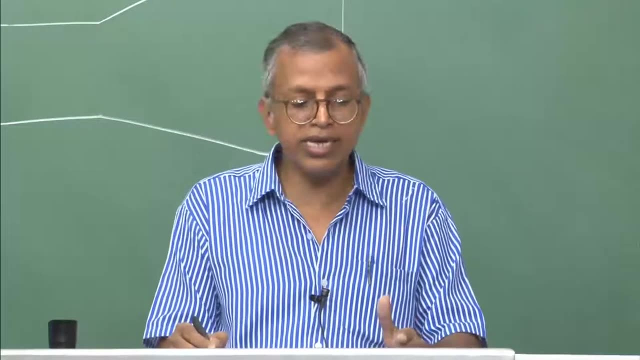 will it depend on the friction or the roughness of the pipe and the material of the pipe? If I want to determine where I can apply the two dimensional equation and one dimensional equation for analysis, that means in this region under developed flow, what is known as all. 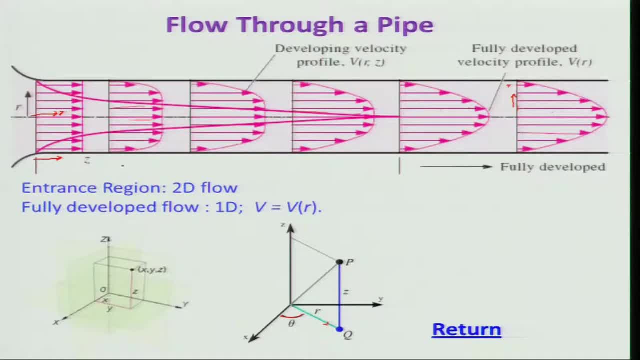 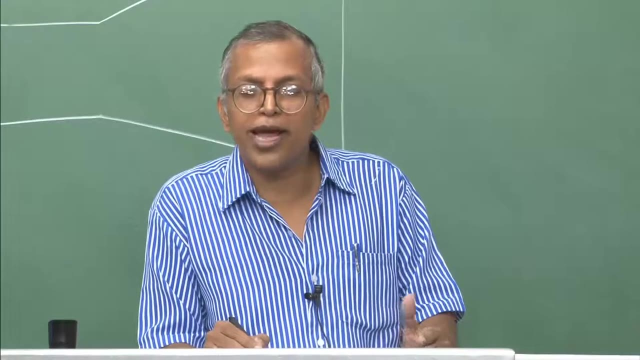 or developing flow. you can say: at this region, from here to here, this region, it is basically call as a developing flow or under developed flow, whatever you call right. I think developing flow is a positive word, like we are developing country. So there what you need to consider. 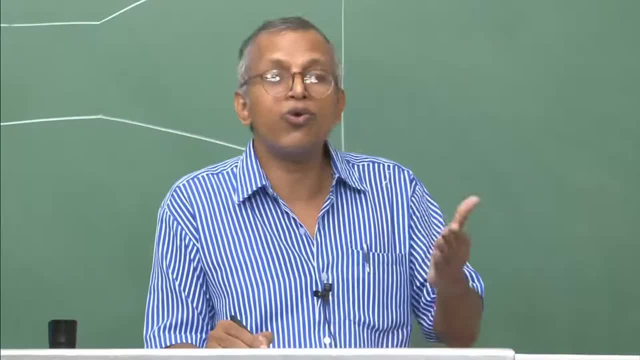 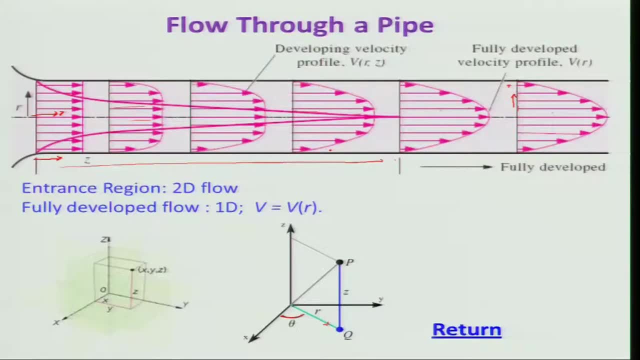 whether the flow will be two dimensional or one dimensional. it will be two dimension. that means So you have to consider the governing equations. that So how well, go about it. it is basically l by d. if I take this, diameter of the pipe for a fully developed flow will be dependent 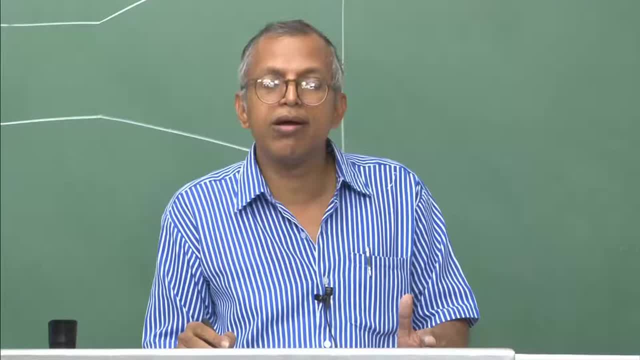 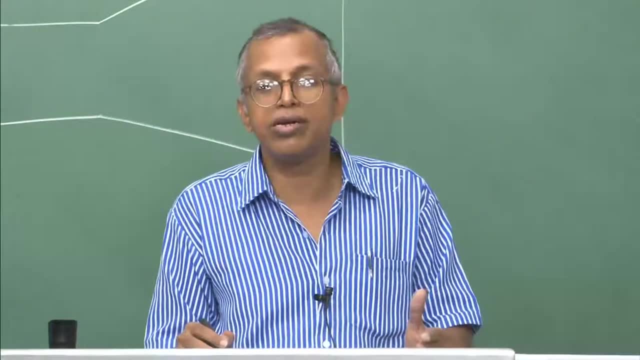 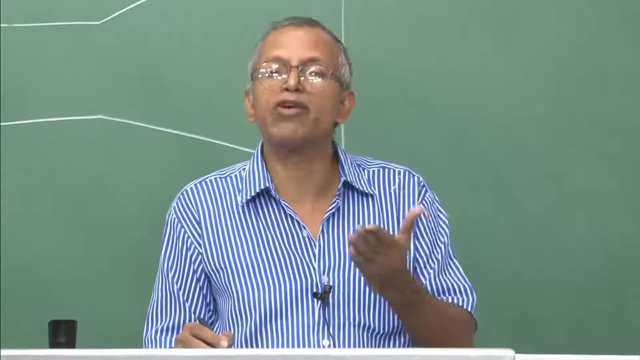 on Reynolds number right. Reynolds number right And for a critical flow. that means where it will go from laminar turbulent l by d for a fully developed flow will be around what? around 125. this is a rough number or a thumb rule you can say. And in case of turbulent, 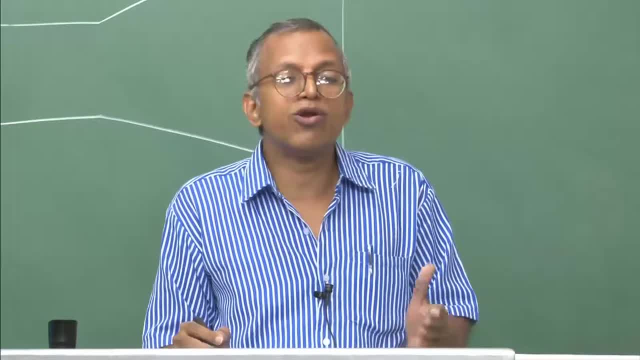 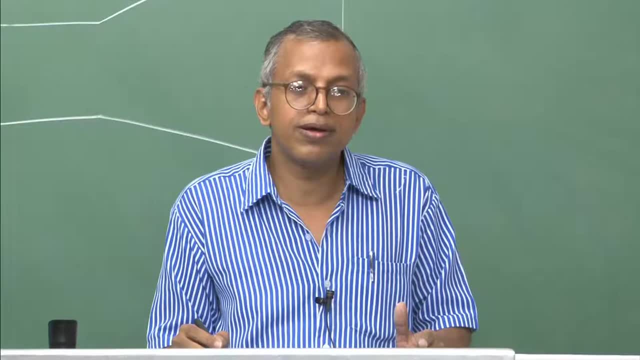 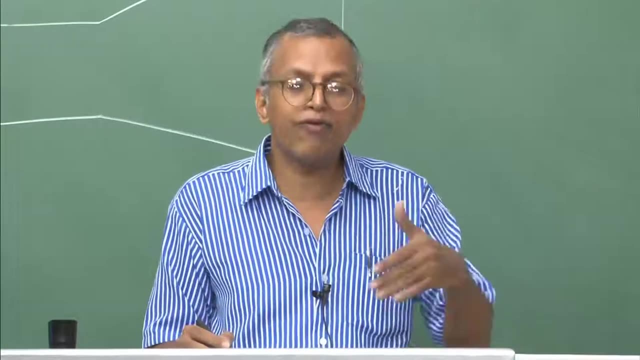 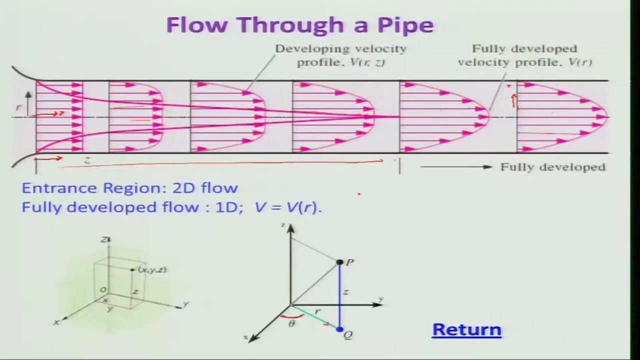 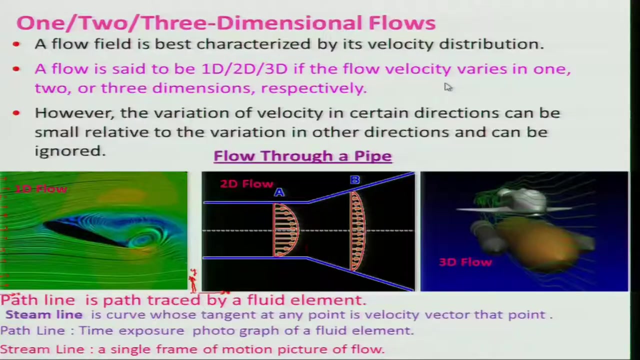 flow. it will take more length to be fully developed for a particular diameter or not, or less. it will be taking less distance, right, And these are very important for analyzing and developing or designing anything. So let us get back to our this thing like a three dimensional flow, right? See, if you? 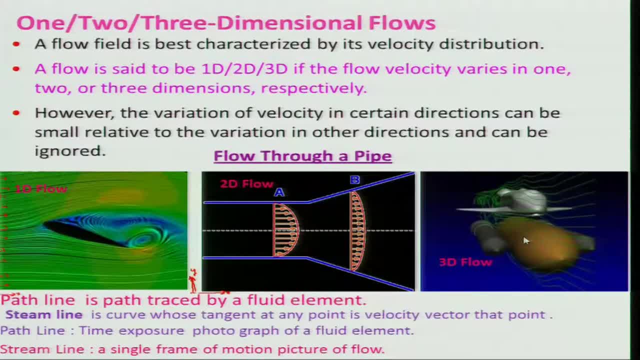 look at flow over a. I have taken a space craft here and you can see these are the lines which indicates it is. you know, you can say this as a path line and if it is a steady flow, as I told, it can be stream line as well. if it is a flow is steady, right. So these lines 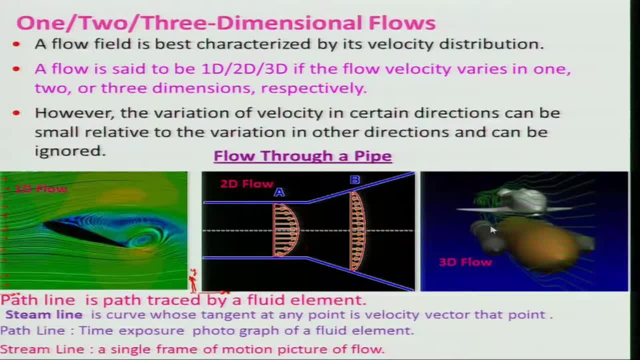 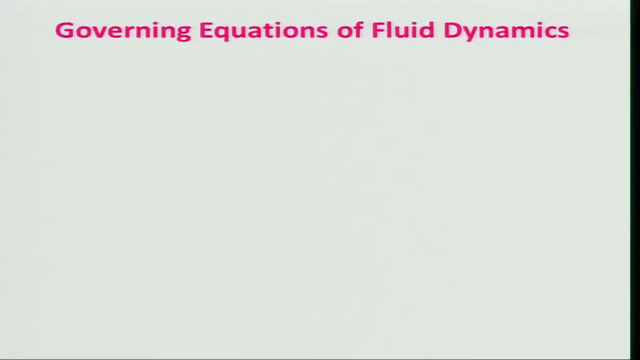 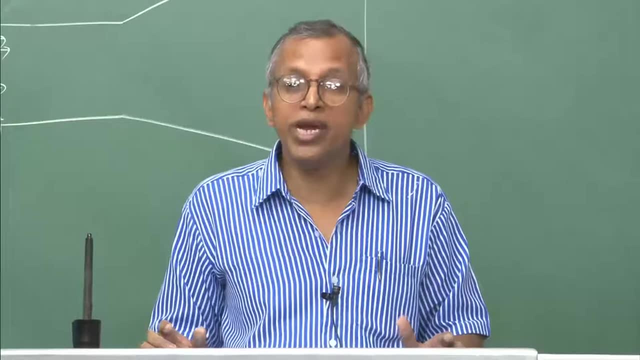 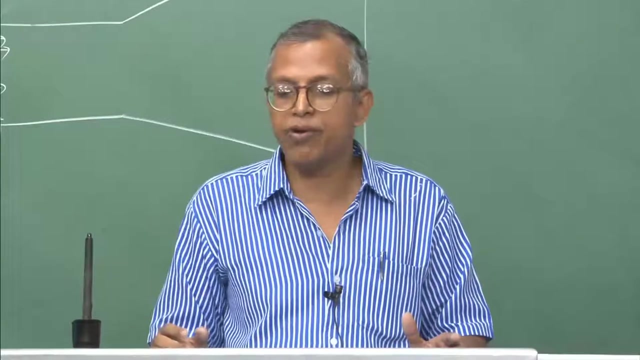 are quite, you know, three dimensional in nature. therefore you can call it as a three dimensional flow. So now we have talked about very what you call qualitatively, about the flow, but we need to now deal with the flow quantitatively, because we will be using this, you know, for 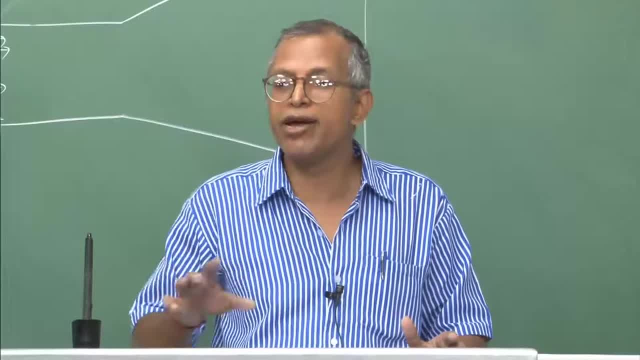 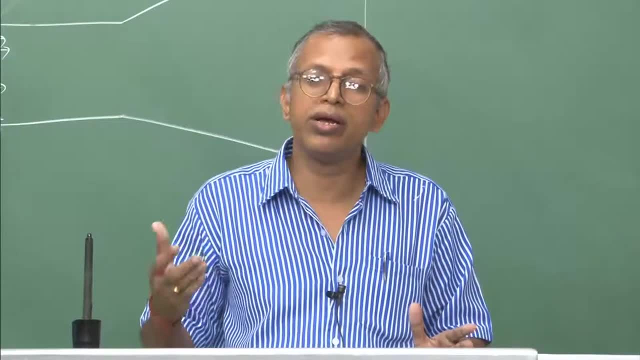 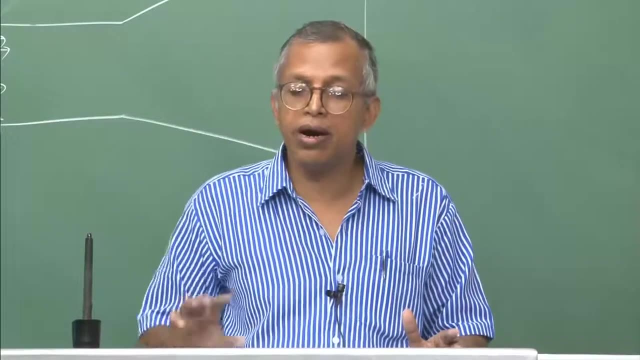 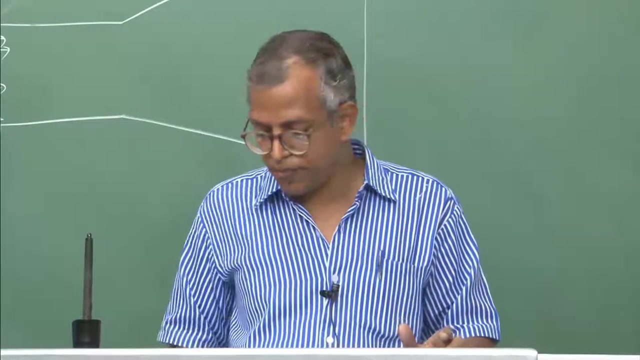 designing certain thing. that means we need to quantify or look at various things. So we will look at various properties. for that we will have to consider the governing equations that will basically dictate how the fluid flow will be there. that means I can really understand or simulate the fluid flow by using certain governing equations. So for that 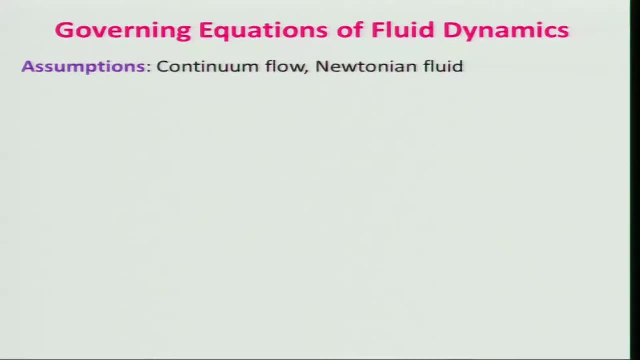 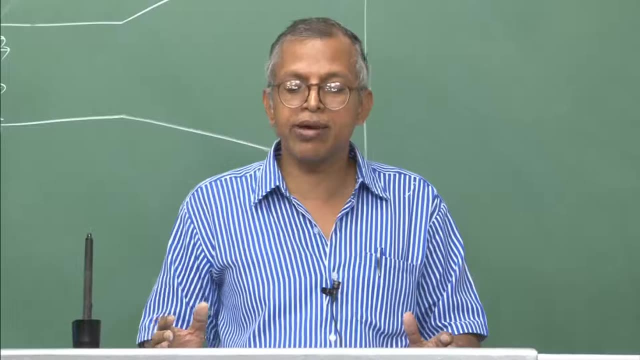 we will make some assumptions. I have already talked about it. what is the continuum flow? that means we will be considering continuum flow in our analysis. So we will make some assumptions. I have already talked about it. what is the continuum flow in our analysis? all the time, except, of course, whenever you go to the space at a very what. 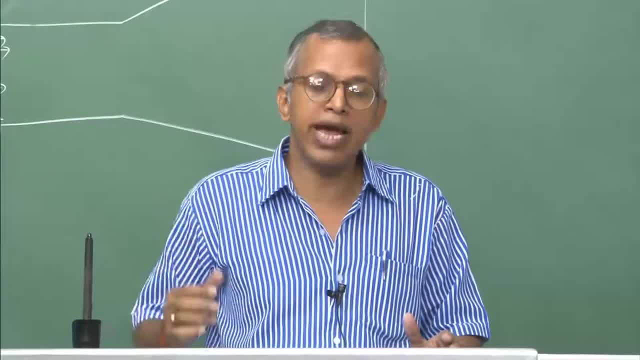 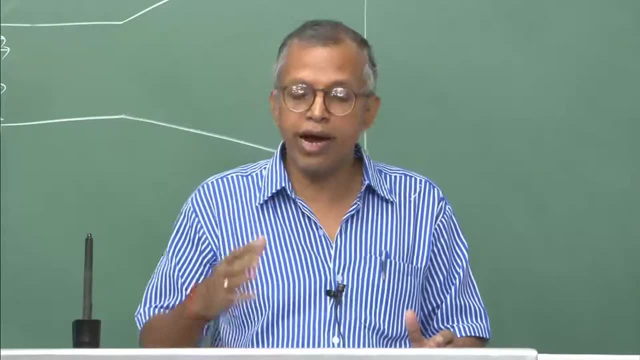 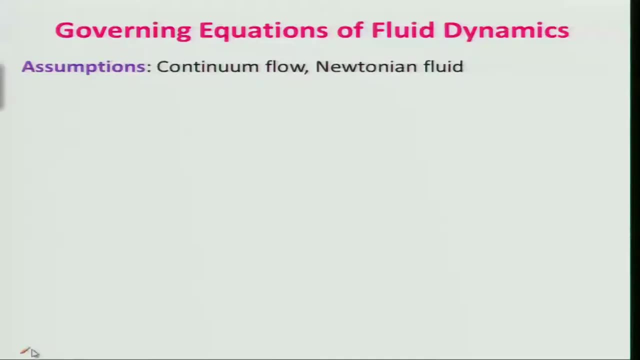 you call low pressure. there the various kinds of flow will be coming into picture, as I told, slip, no slip flow and then free molecular flow kind of things. but we are not bother about that and, as I told, we will be considering basically about the Newtonian fluid. So we 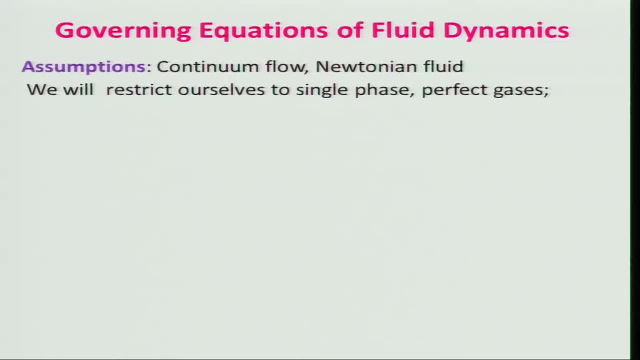 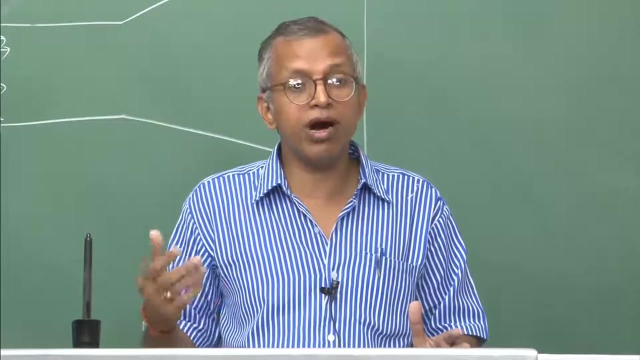 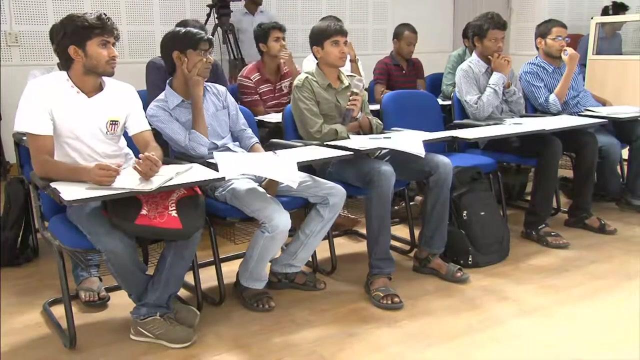 will discuss to a single phase fluid and as we are dealing with the mostly the gases, then we will be considering as a perfect gas. what do you mean by perfect gas? No reaction takes place. No reaction takes place. we call it as a perfect gas. can anybody tell me, please, what do you mean by a perfect gas? 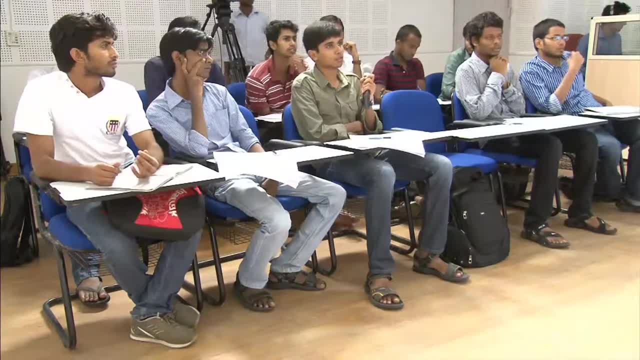 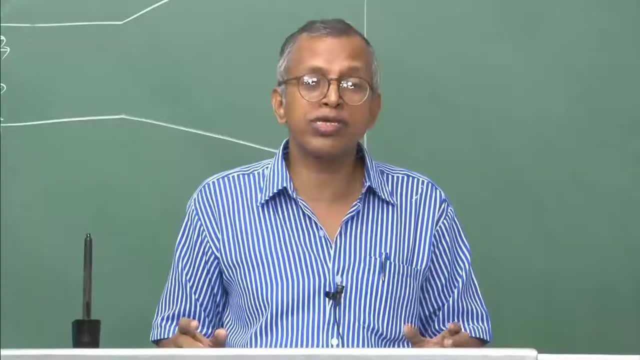 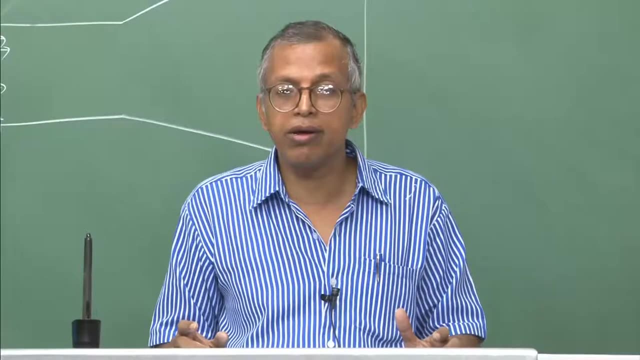 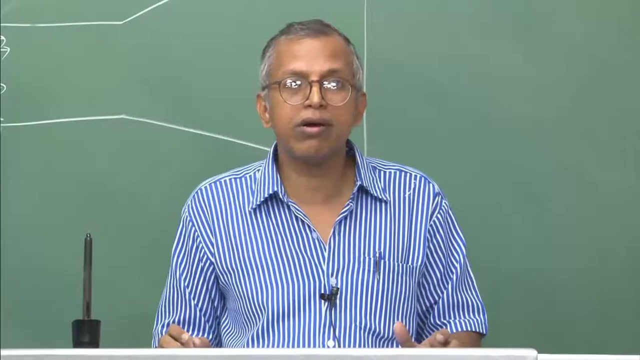 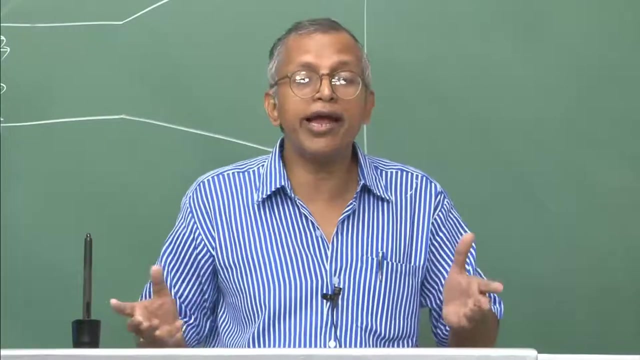 That means in the molecular forces between or among them in a gas, will be very, very small when it will occur. when it will occur, this inter molecular forces will be less. it can occur only when the pressure will be low. what kind of low which can tell what can happen? 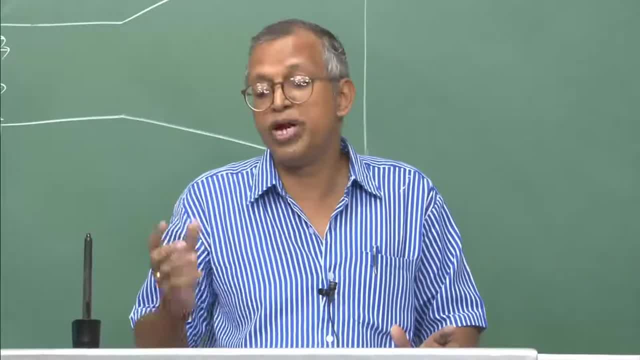 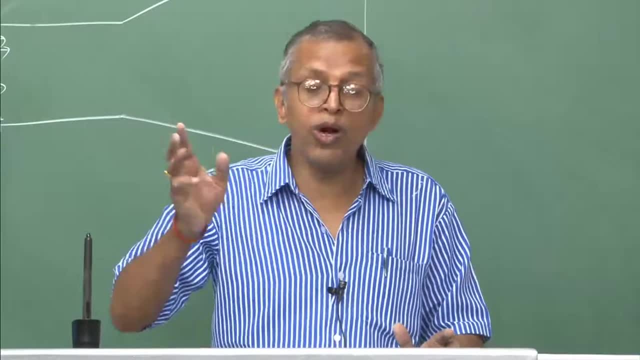 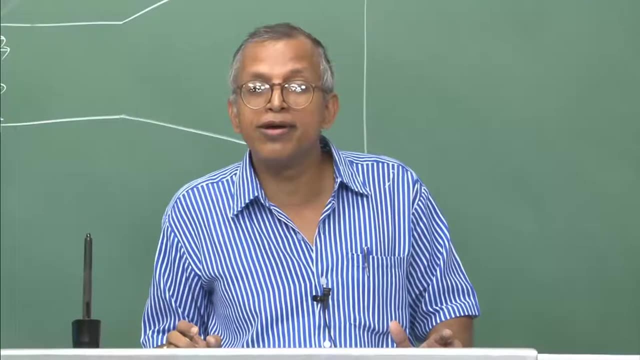 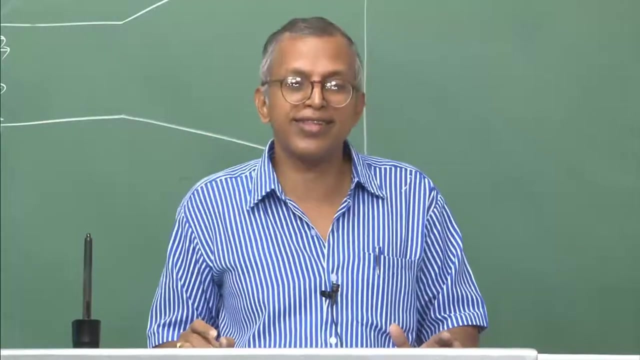 tell us that, whether the flow is, or the fluid is perfect or not, or gas is the perfect or not. Is it the only condition or there is some another condition which will tell you whether the gas is perfect or not? The volume occupied by individual particles or the molecules? 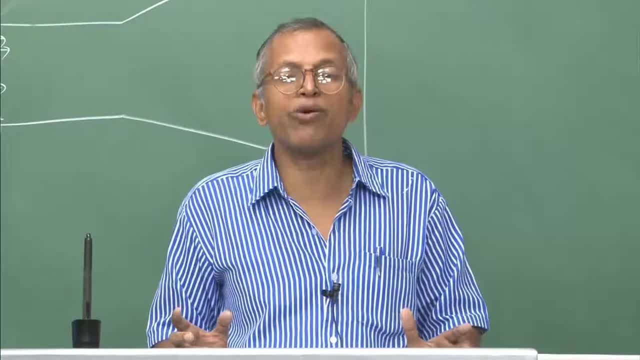 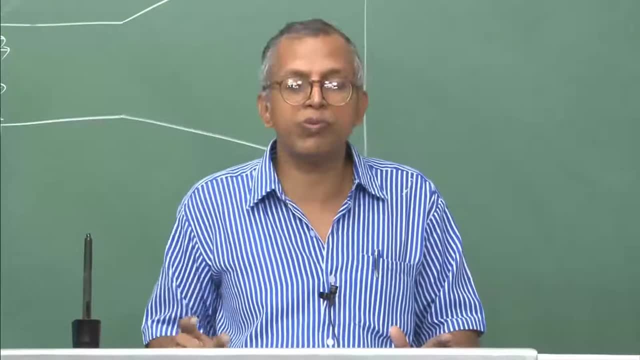 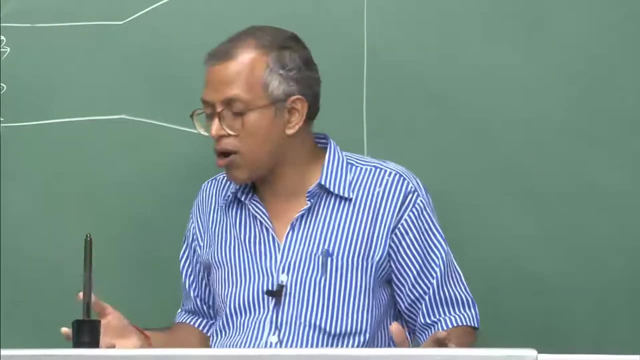 will be quite less as compared to the volume of the fluid, which will be considered right Then only if both this condition satisfied, then only one can call it as a perfect gas. and where ideal gas law p v is equal to n, r, t will be right. Yes, it will be, but then 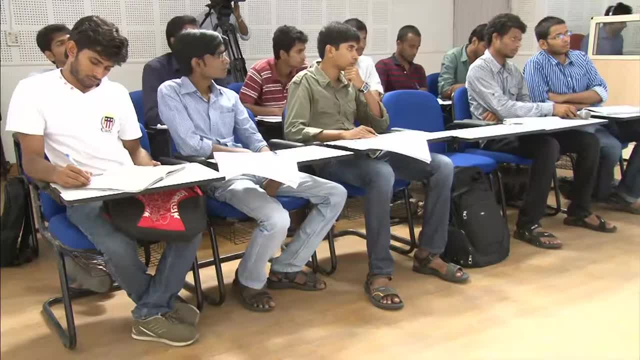 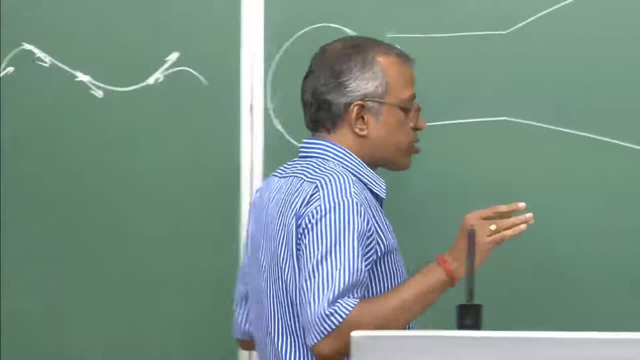 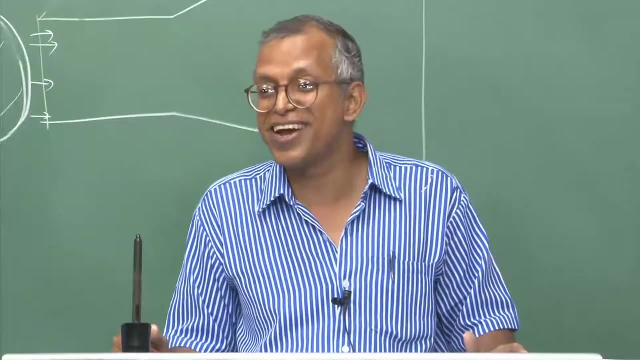 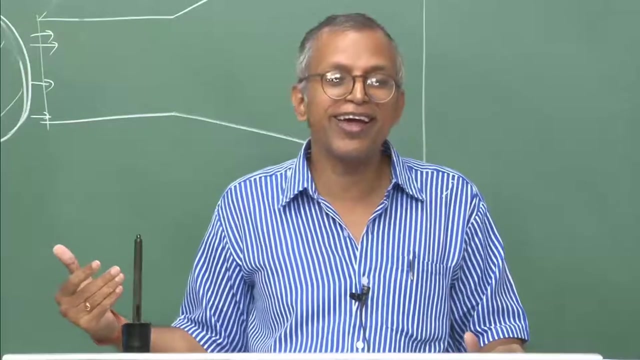 that connotation will be little different. perfect liquid will be there when you call about, you know. So, here, when you are saying perfect- actually this perfect is not a good word as such. right, because you know we are saying it- is we satisfying a simplified form of equation state what is? 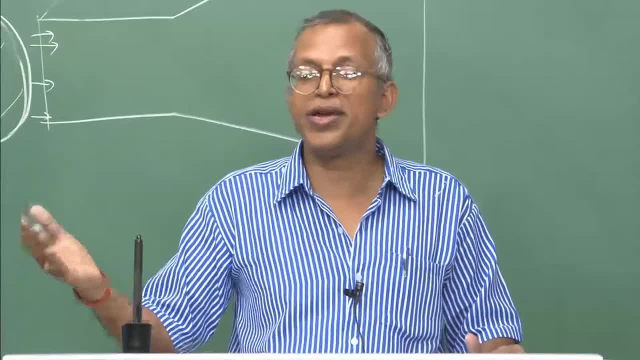 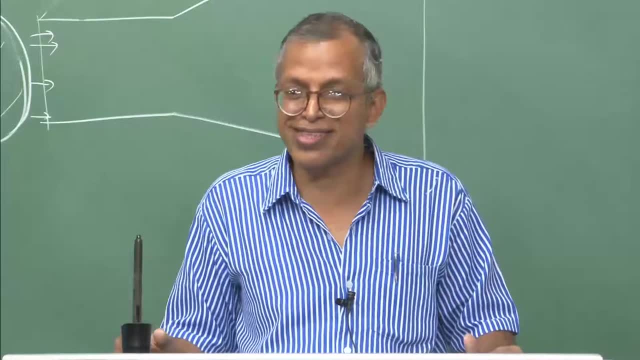 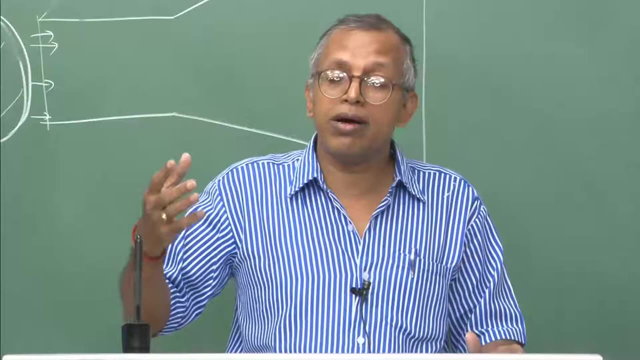 known as ideal gas law. right, Then we are calling it as a perfect gas. actually, I will say that is a Rather. this is an imperfect gas according to my version, but people are saying we will have to go by that word, naturally. but the question is that, like what we will call at, 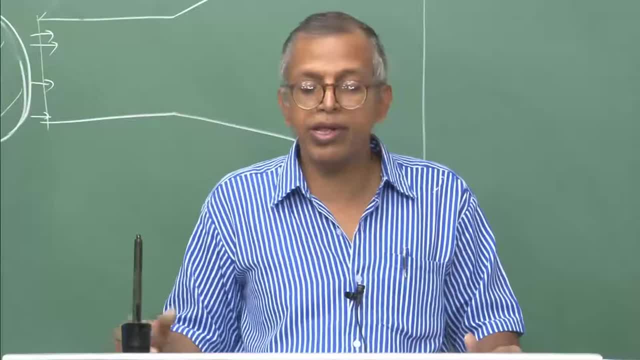 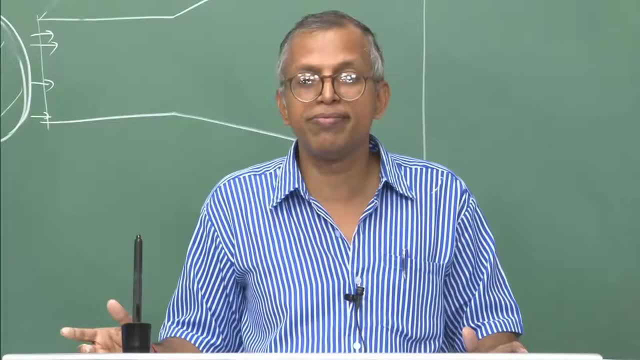 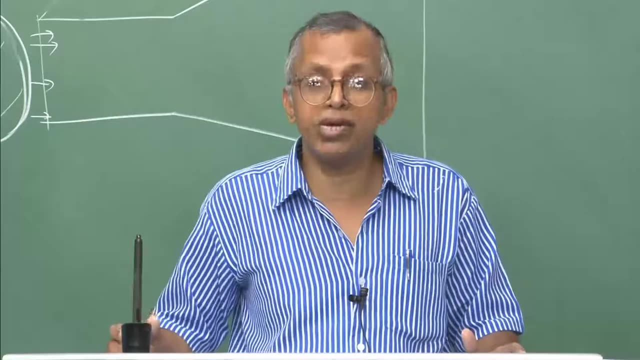 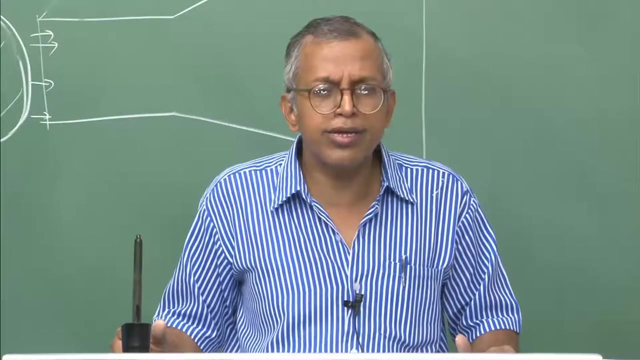 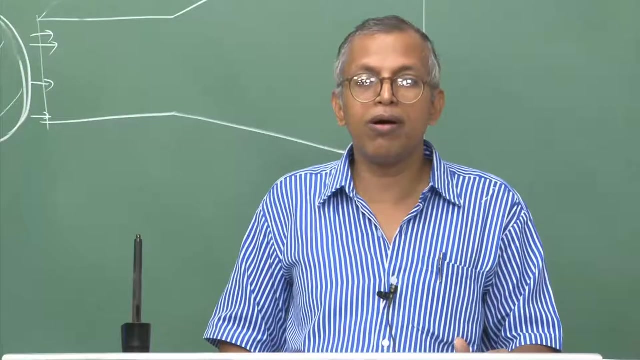 what pressure, what temperature we can talk about, whether the flow is perfect or not, or whether it will follow the ideal gas or not, law or not. Is it? if I take ambient pressure in a air in this room, let us say at a ambient temperature, can you call it as in a perfect gas and then apply the ideal gas law, yes or no? but I want. 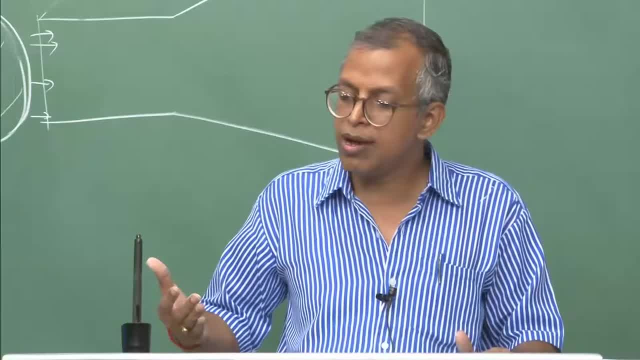 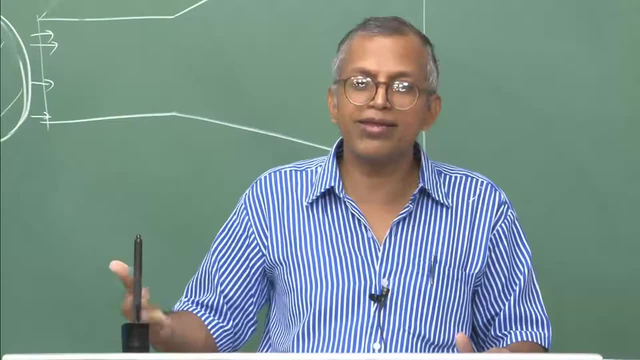 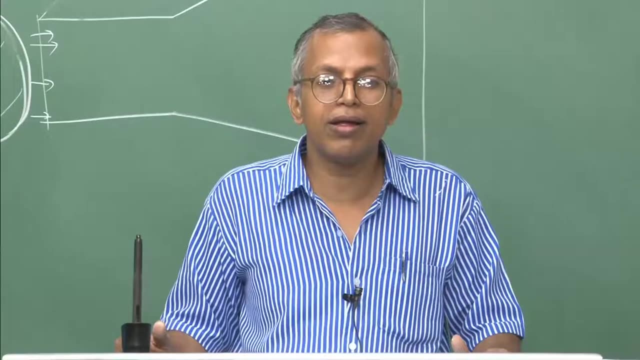 answer. you know all those things. this you are learning from your class, I think may be tenth onwards- ideal gas law is being taught, I think right, And then what is the ideal gas law? What is the ideal gas law? And you are being engineering already, so you are, you know all these things, right.